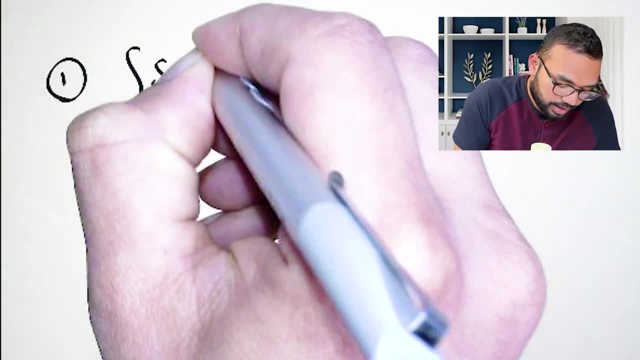 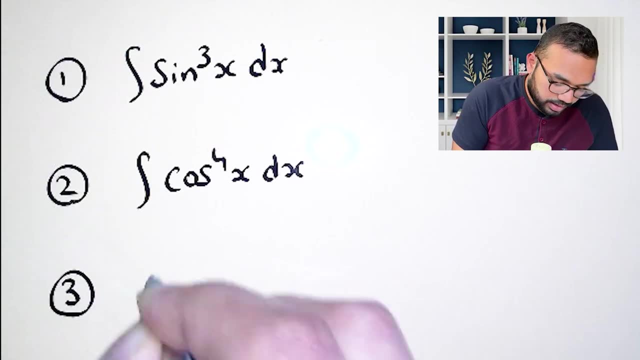 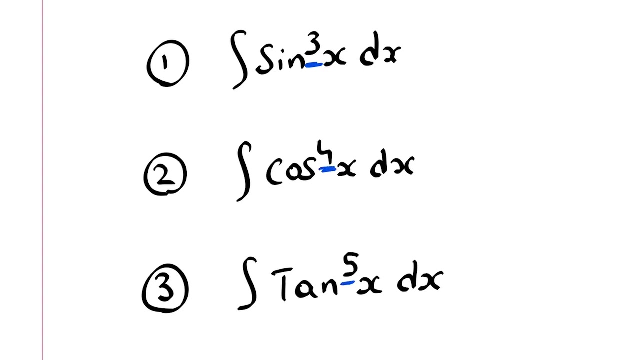 Here are some simple examples: Integral of sine cube x dx. Integral of cos power 4 x dx. And integral of tan to the power of 5 x dx. If you observe, I chose the integrands with odd powers and even powers Because the technique of integrating odd powers of trigonometric functions 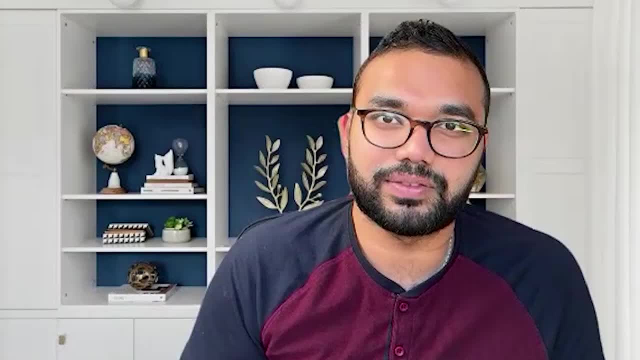 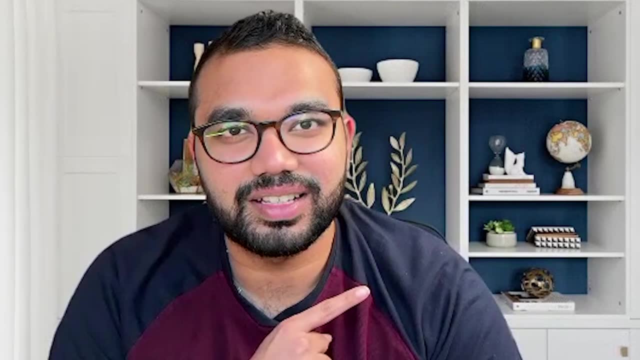 and even powers of trigonometric function is going to be a little different. If you don't know what is an integrand check out my previous video. It is going to be displayed right over here. Please check it out. Alright, let's get back into the video. 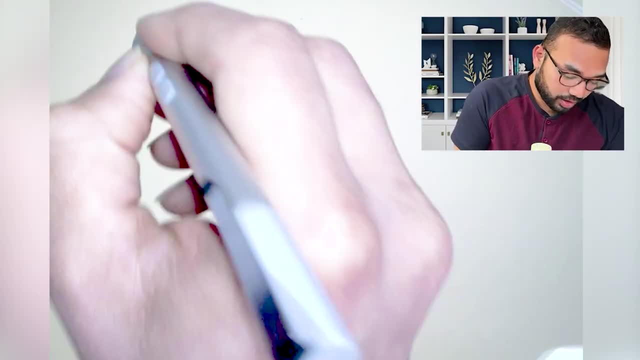 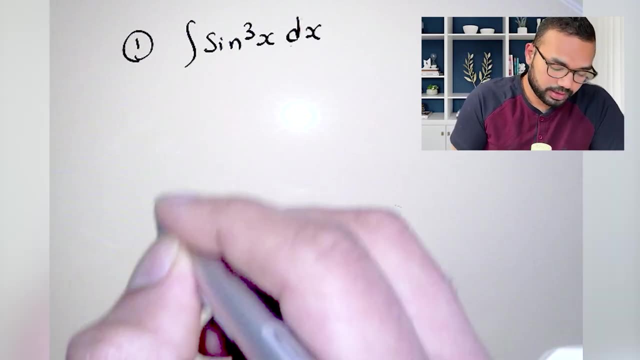 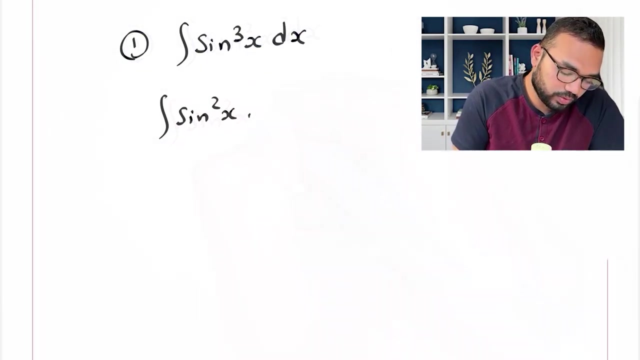 Let's solve our first problem, which is integral of sine cube x dx. The way I would solve is first split this sine cube x as integral sine square x into sine x dx. I know that derivative of cos x- dx is integral of sin x dx. I know that derivative of cos x- dx is integral of sin x dx. So I try to calculate the conjugal of sine cube x and x by i and find out also by multiplying the integral of sine x and x into sin x, dx. Let's take the length of sine x and x. P is equal to sweet prime of x divided by the integral of sine x. 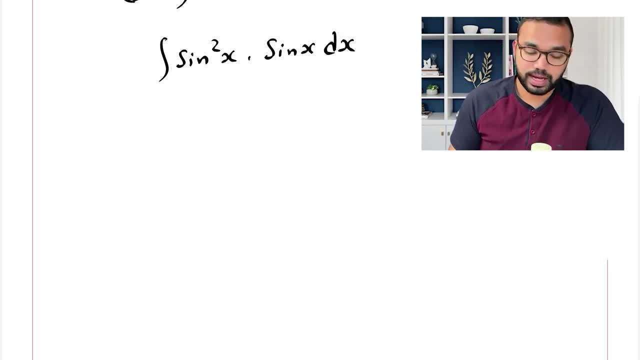 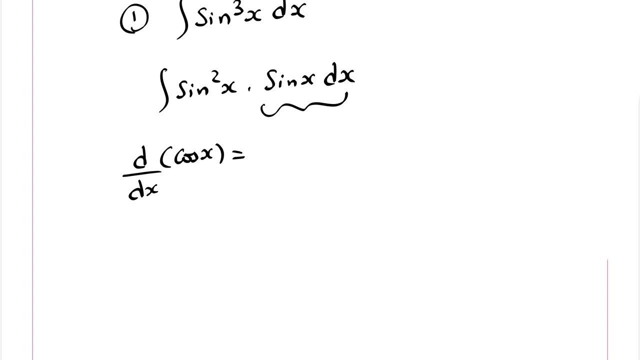 So P is equal to sine x and x, and this one equals the length of the connection of sine x plus sine x and y. Right, In the case of the integral of sine x, we have 2 twin powers on the square, and 4 say that sin x- dx or sin x- dx sale up. 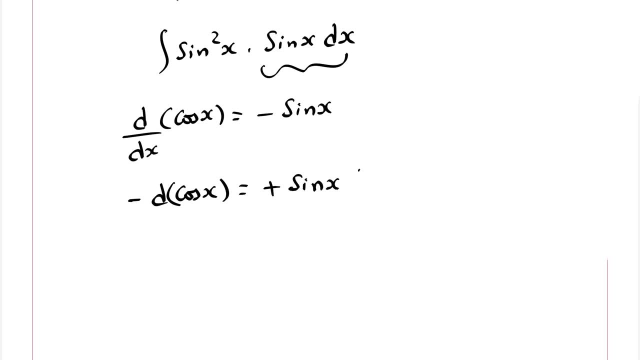 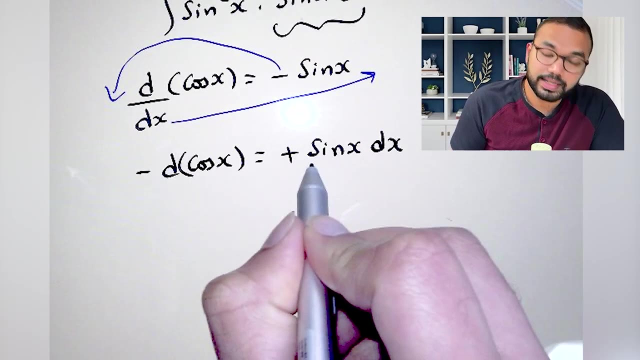 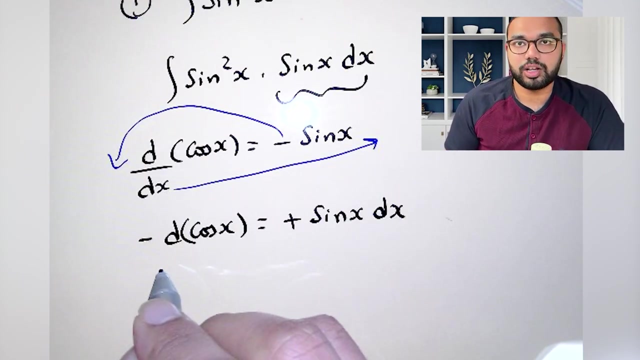 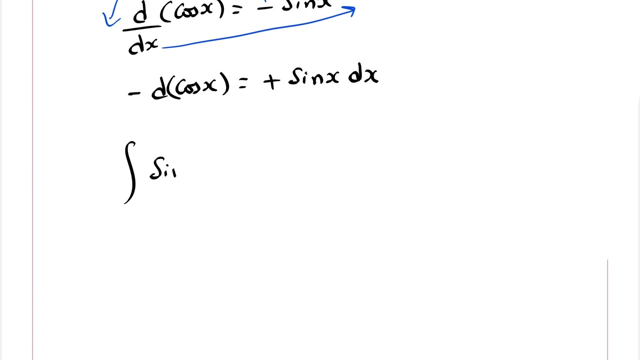 to positive sine x dx. what i just did is basically bring this dx here and minus sine over here. so minus d of cos x is sine x dx, right. so i'm going to plug this for sine x dx. i'm going to plug minus d cos x for sine x dx right. integral of sine square x. minus d of cos x, minus integral. 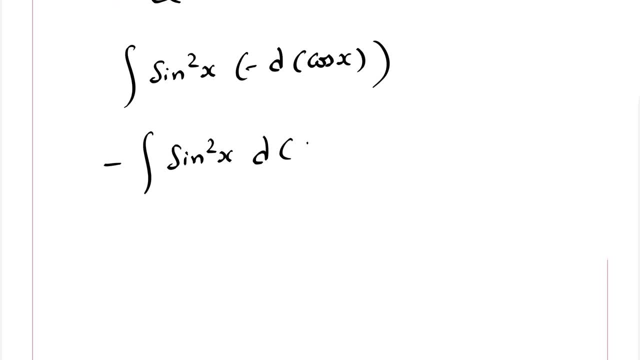 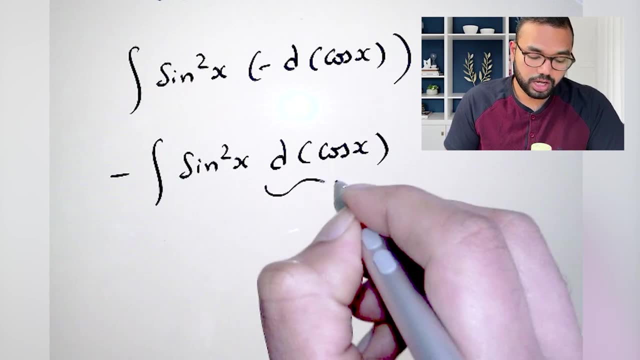 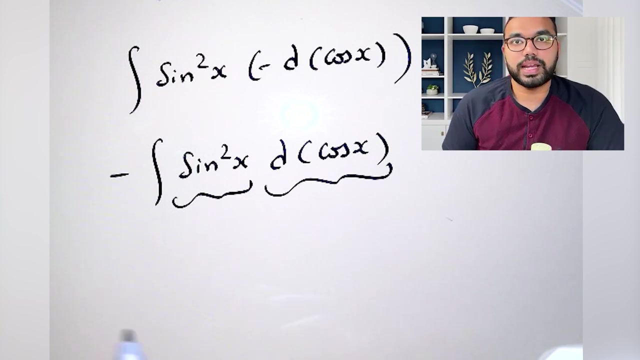 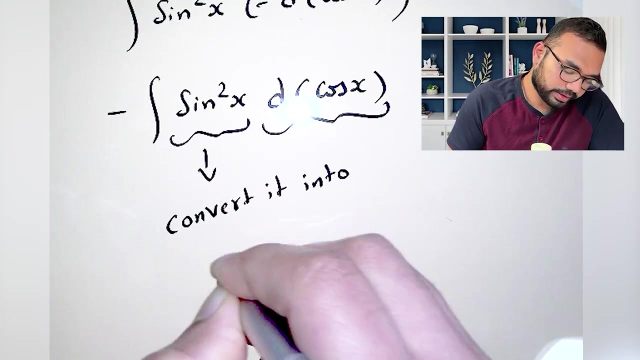 sine square x, d of cos x. so now my differential is d of cos x and the integrand is sine square x. so i need to convert my integrand in terms of differential. so that means i have to convert sine square x in terms of cosine, so convert it into cos. i will use the trigonometric identity. 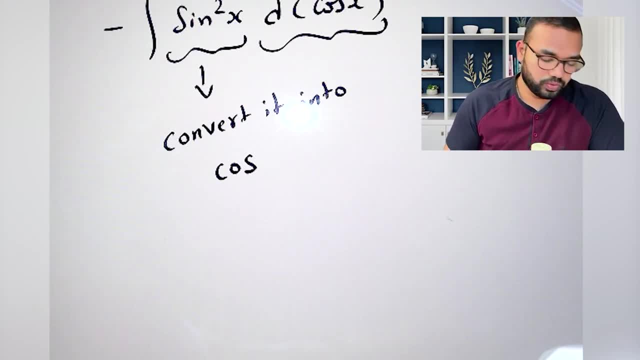 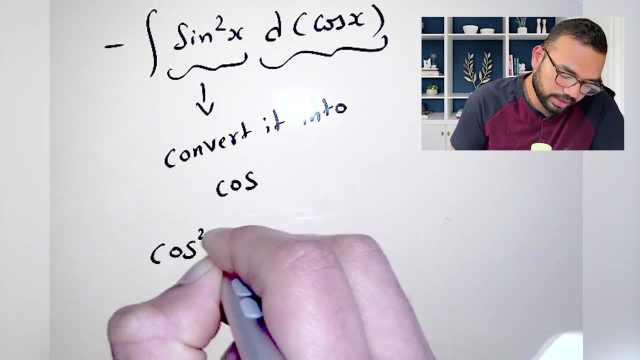 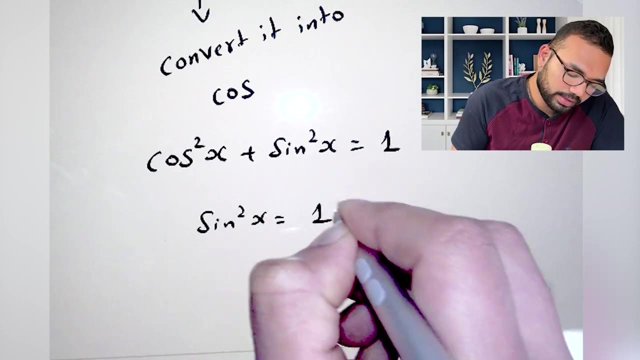 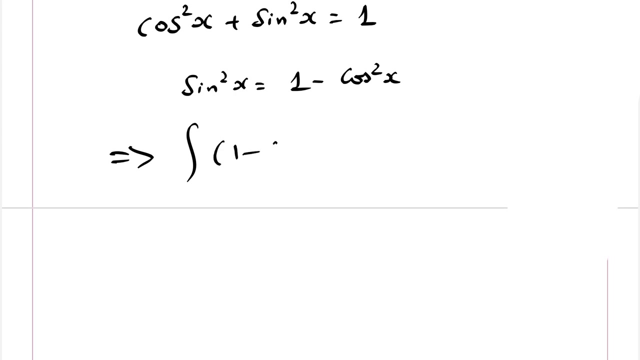 cos square x plus sine square x is equals to 1, right, so i can write: cos square x plus sine sine square x is equals to 1.. So sine square x is 1 minus cos square x. Therefore our integrand is 1 minus cos square x. b of cos x and negative symbol over here. So just: 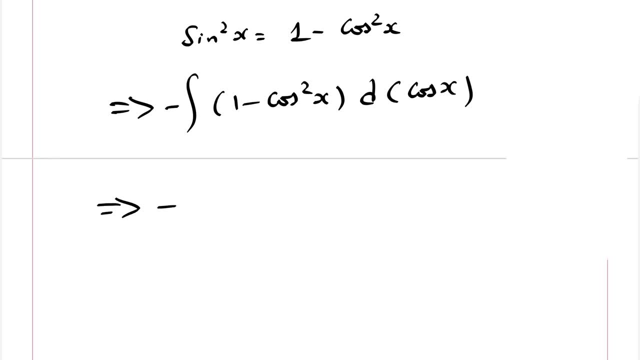 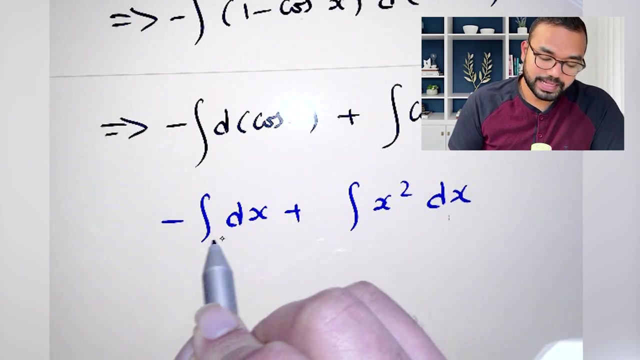 distribute this differential all over: Minus b of cos x plus integral cos square x b of cos x. Isn't this looking like our standard formulas? Minus integral dx plus integral x square dx? Right, But we just have cos x. We know how to integrate dx and integral x square dx. 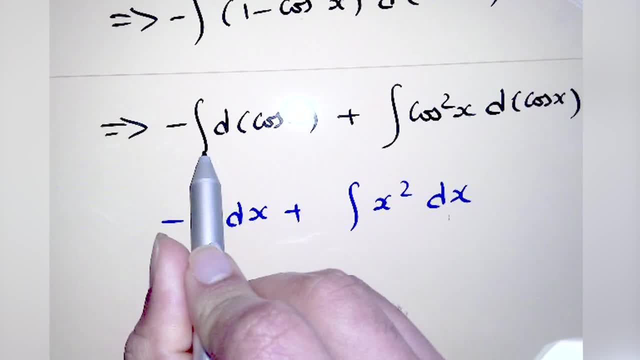 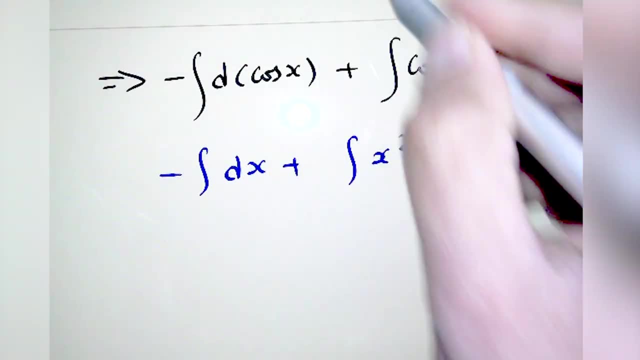 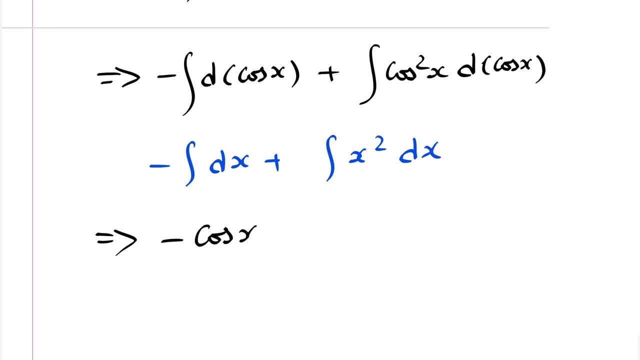 In the same way, we can integrate d of cos x and cos square d of cos x. So what do you think is our final answer? It is going to be minus cos x, minus plus cos cube x, divided by 3, plus integration constant c. This is going to be our final. 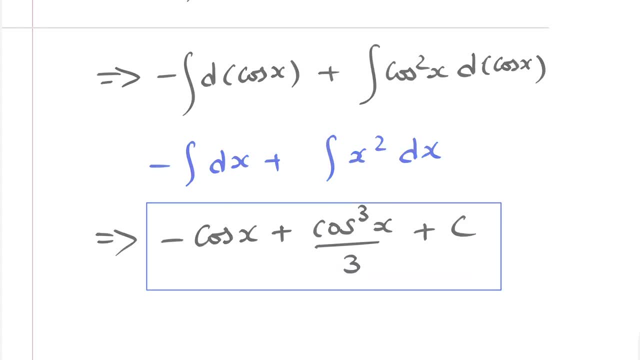 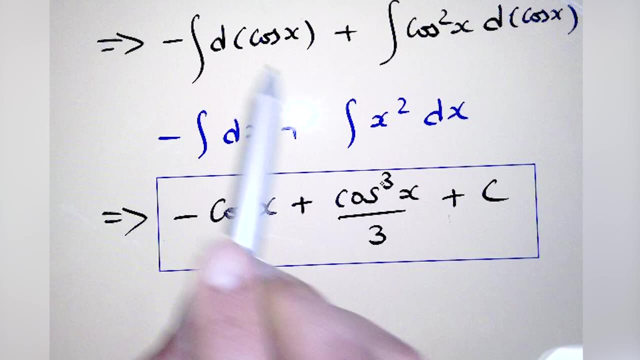 answer: Because integral dx is x, integral x, square dx is x cubed by 3.. So since we have d of cos x for our differential, we're going to write in terms of dx and integral of cos x minus cos x plus cos cube x divided by 3, plus integration constant. 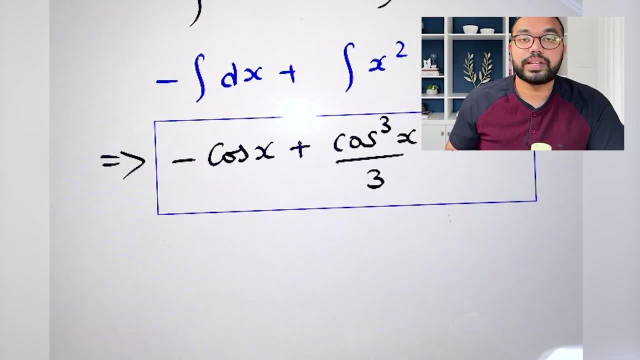 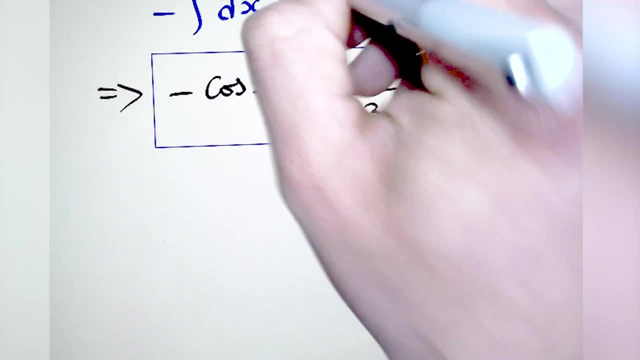 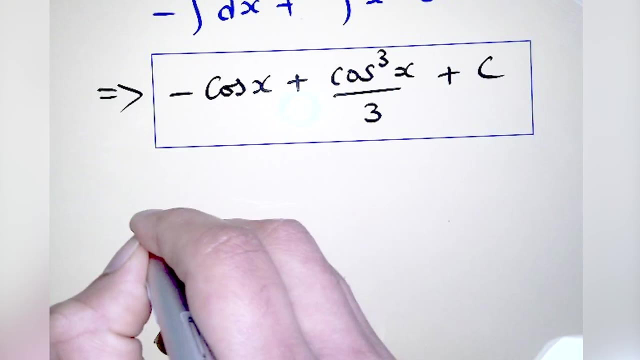 Now, if we want to verify our answer, we can do one thing. We can derive this final answer to get our integrand function sine cube x. So if I derive cos x, it is going to be minus cos x, So it is. 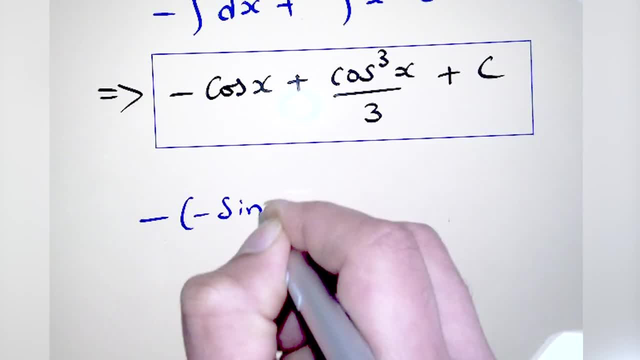 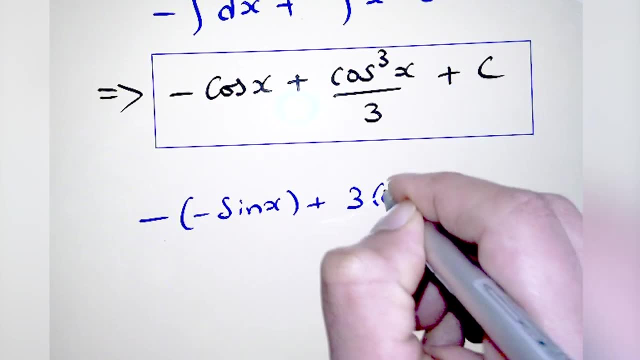 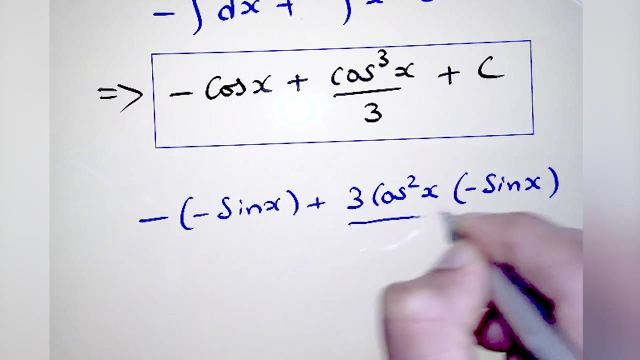 minus half, minus sine x, and cos cube x derivative is 3, cos square x and derivative of cos x is minus sine x, because this is a chain rule divided by 3 and integration of constant is simply 0. So I'm not going to write. 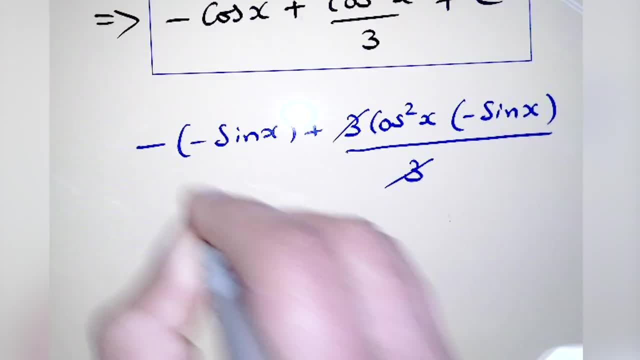 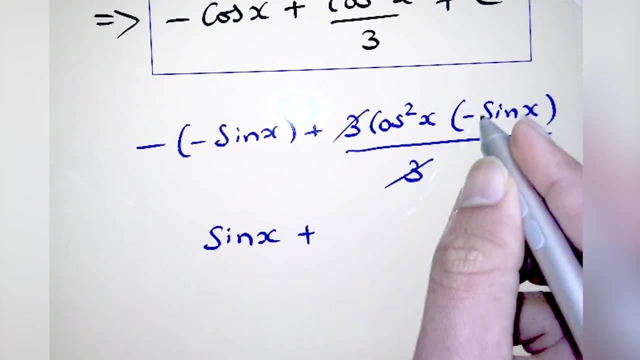 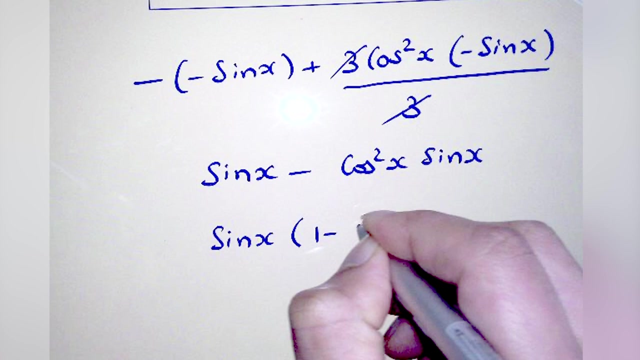 that. So 3 and 3 would get cancelled. Negative times negative is sine x plus and the sine in between is minus. So minus cos square x into sine x. I can take sine x common Sine x, common sine x of 1, minus cos square x, So sine x. 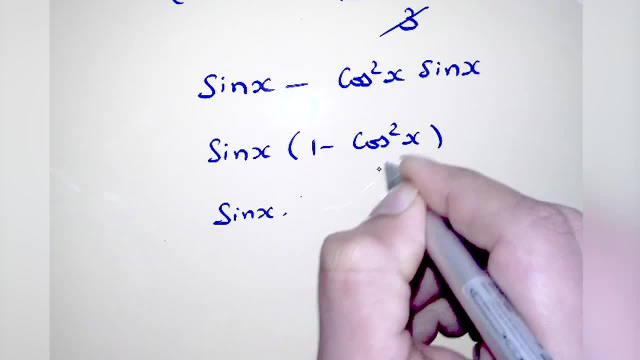 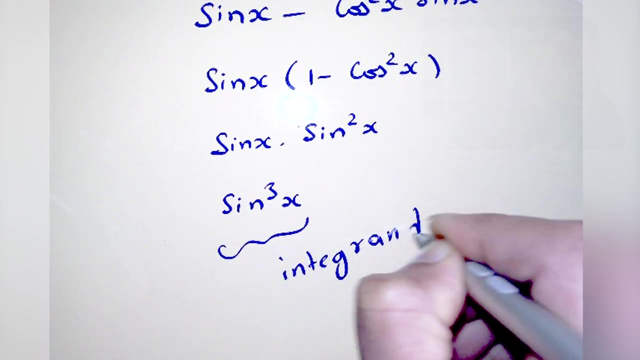 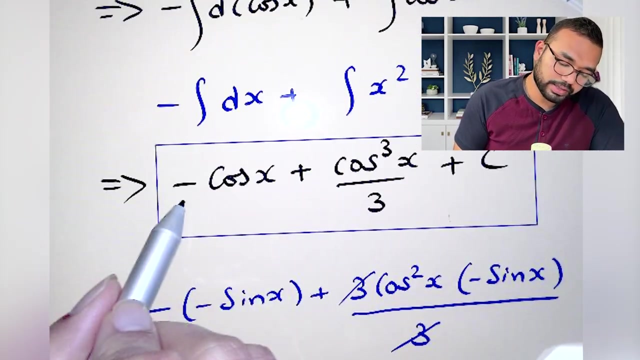 to 1 minus cos square x is sine square x and this is sine q. This is our initial integrand. So we got our integrand and I derived the answer. So this says that our answer, minus cos x, plus cos cube x divided by 3 plus c, is the correct answer. 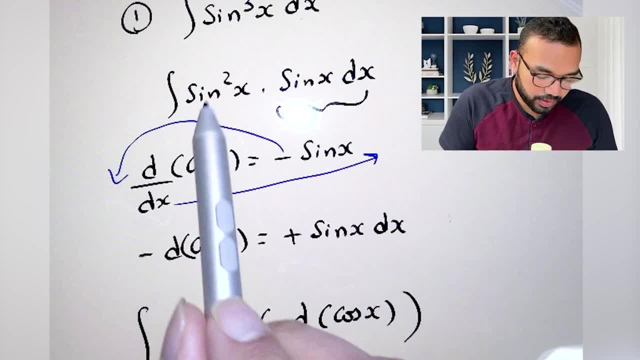 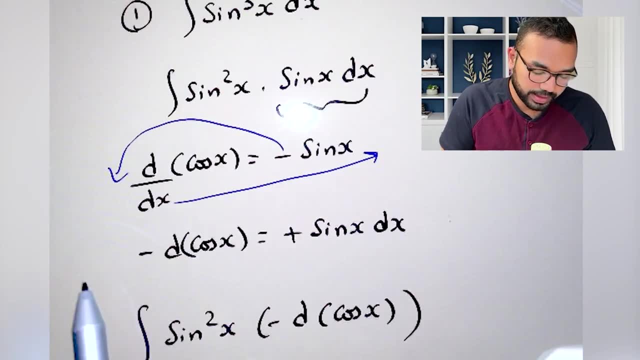 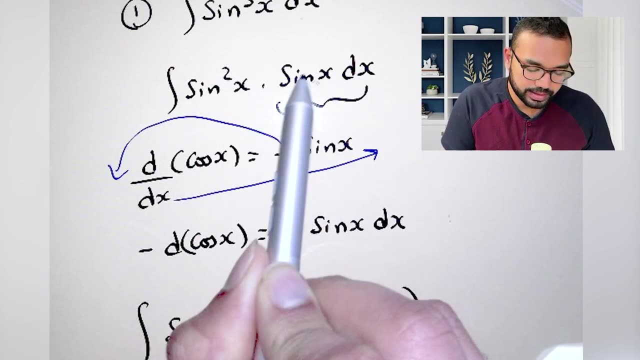 Let's summarize what we just did. So our problem is to integrate sine cube x with respect to x. So the first step I did is to split this odd power into 1- even power and sine x- dx- Even power into sine x- dx. So I know that I can write this sine x- dx as: 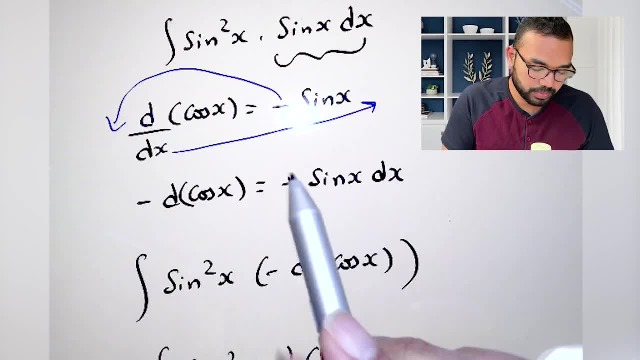 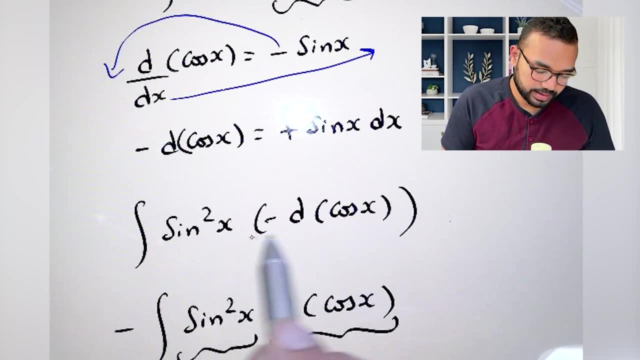 d of cos x. So sine x dx will be minus d of cos x and you can plug that for sine x dx. So I just did integral of sine square x Times minus of d of cos x. So I brought the negative sign outside of the integral. 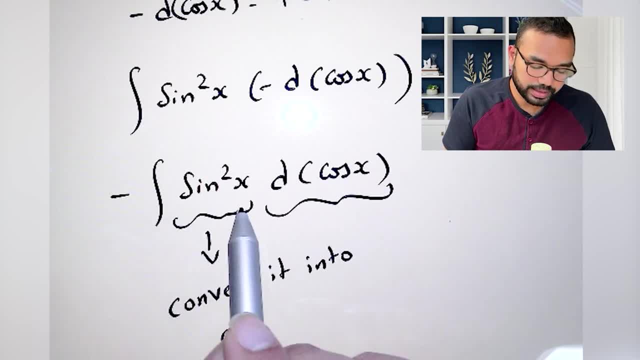 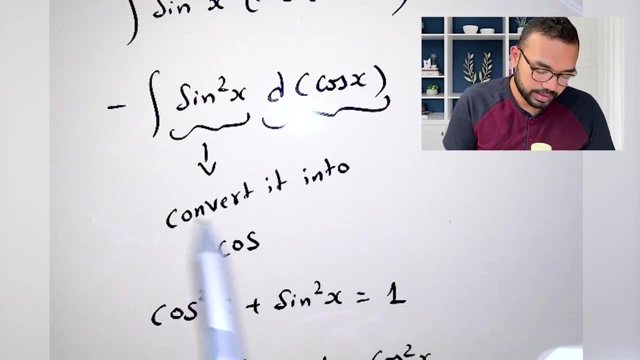 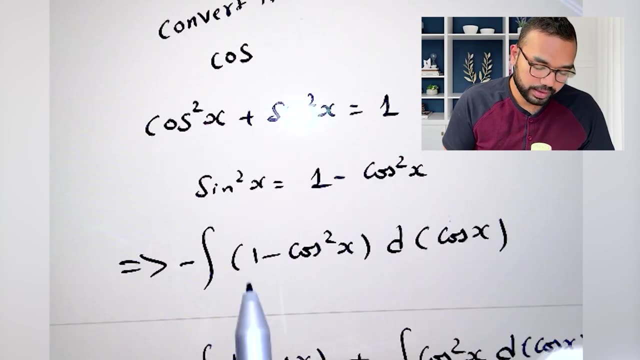 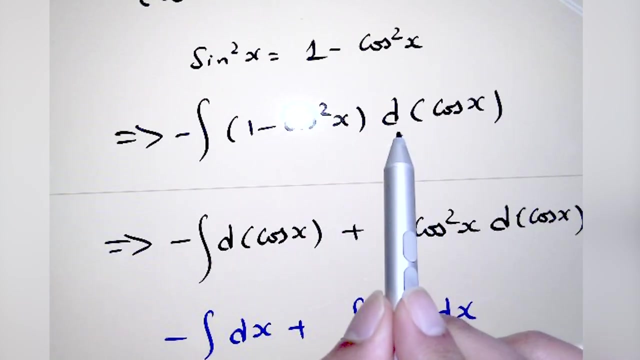 So it is integral sine square x d of cos x. The next step: I converted this sine square x in terms of cos using the trigonometric identity. So I have written 1 minus cos square x for sine square x And I distributed the differential d of cos x minus integral d of cos x plus cos square x d of cos x. 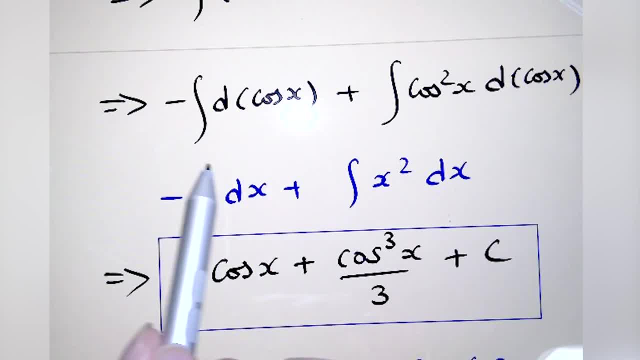 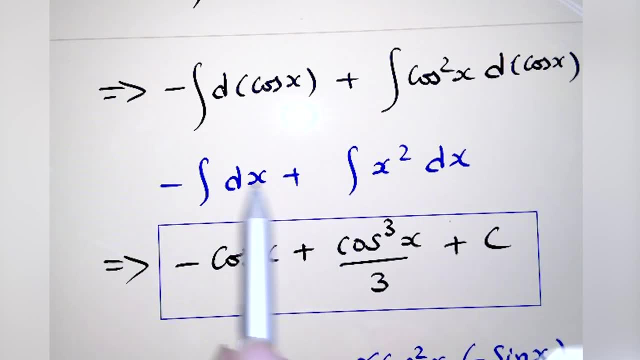 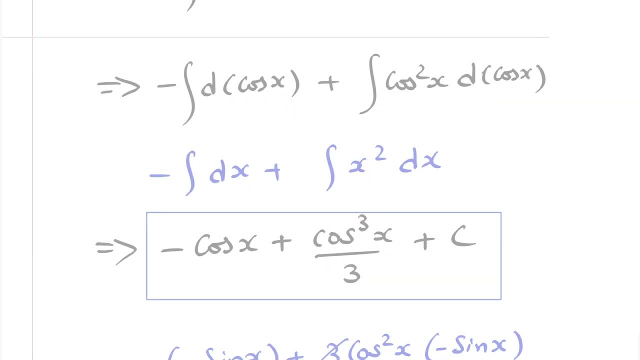 And this is just looking like our integral dx and integral x square dx. So we can apply our standard formulas, But we will just use cos x for x. so final answer would be: minus cos X plus cos cube X by 3 plus C. right now. 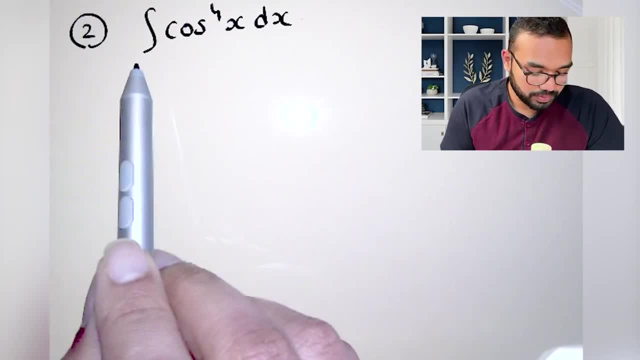 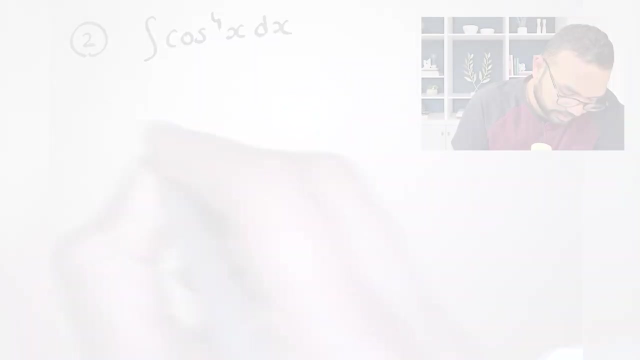 let's move on to the second problem: integral cos power 4x DX. the method to integrate an even power is slightly different than an odd power. you will see the difference. so the way that I would do is I can write cos square X in terms of cos 2x as cos 2x plus 1 divided by 2, right? so what will happen to cos power? 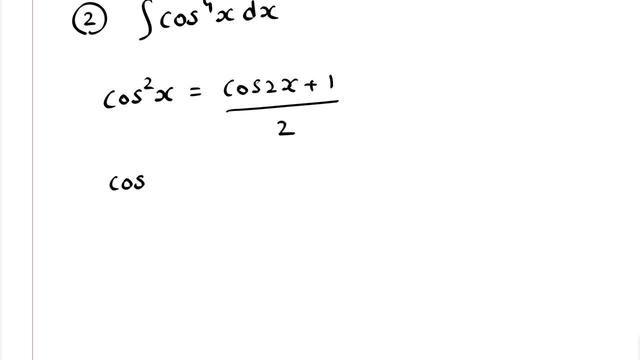 4x cos power 4x is simply cos square X, whole square. so cos 2x is equal to cos square X, whole square and what will happen is it will cos power 4x is going to be cos 2x plus 1 by 2 whole square. So if I square the numerator, 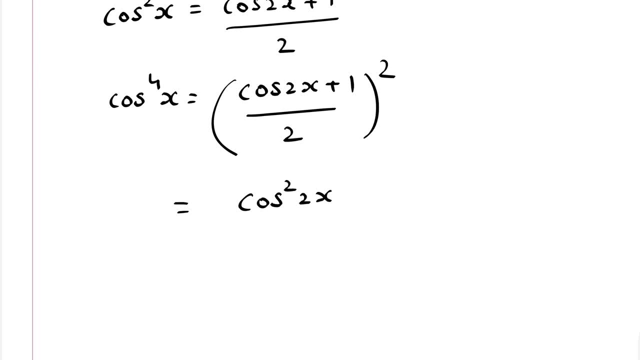 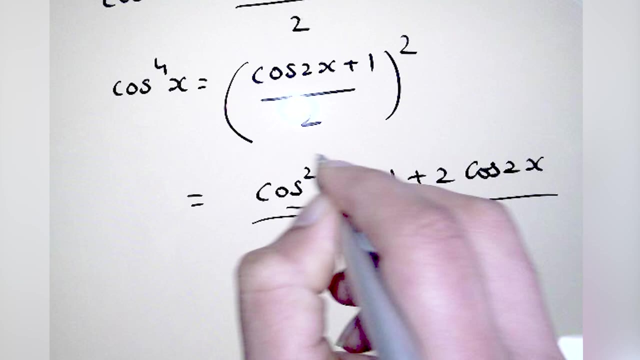 it is going to be cos square 2x plus 1 plus 2 times cos 2x divided by 2 square is 4.. I still have this cos square 2x. I don't want any squares or fourth powers, I just want. 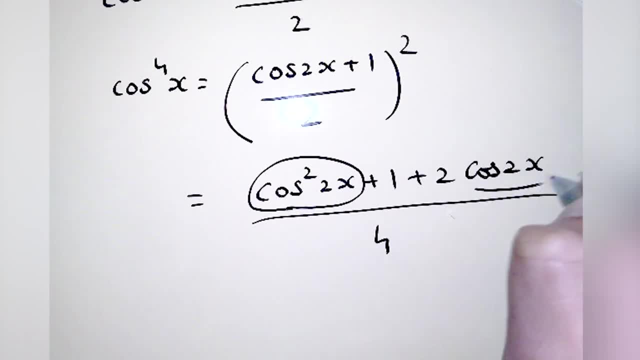 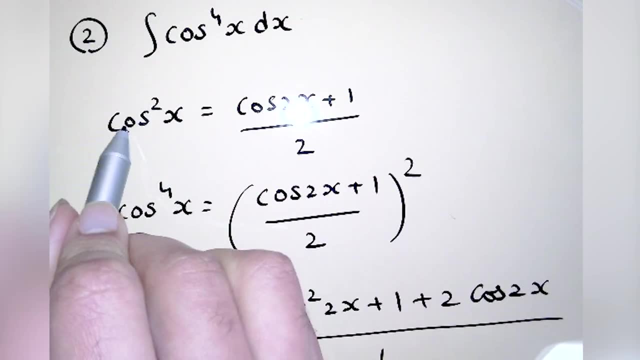 like this, our ones like cos 2x. So what I'm going to do is apply this formula, same formula again, but write: cos square 2x is equals to cos 4x plus 1 by 2.. So 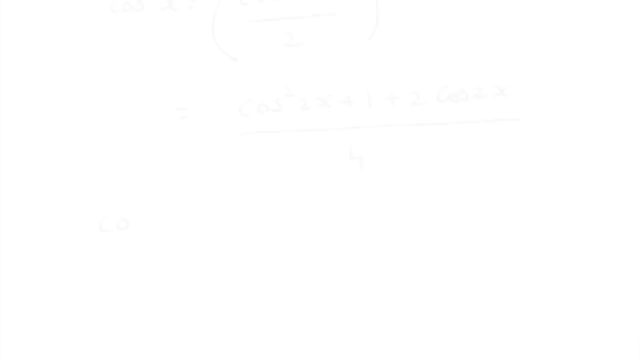 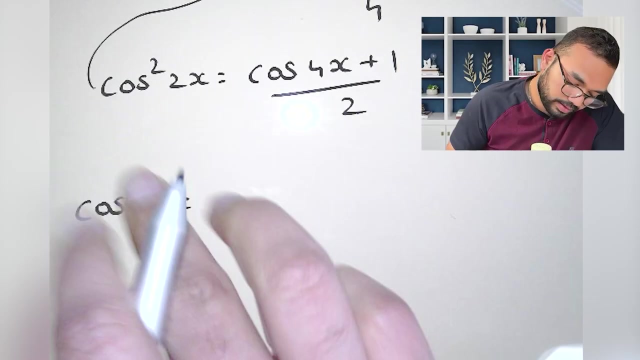 let's just apply. Let's apply that here: So cos square 2x is cos 4x plus 1 over 2.. And I will plug this over here. So cos power 4x is so cos 4x plus 1 by 2.. 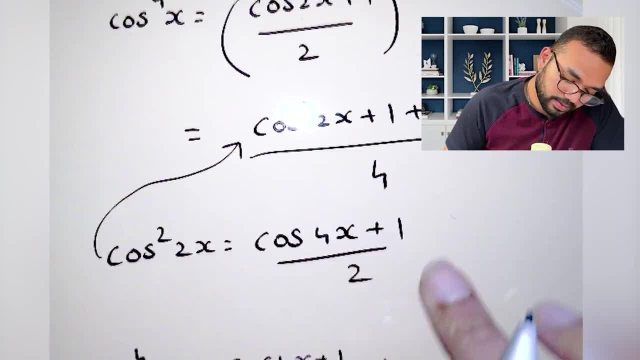 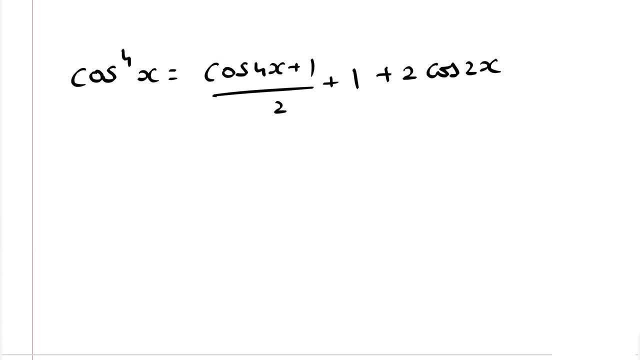 And I will plug this over here. So cos square 2x is so cos square 2x plus 1 by 2.. So and whole divided by 4. If I simplify this, it is going to be cos 4x plus 1 plus 2 plus 4 cos 2x. 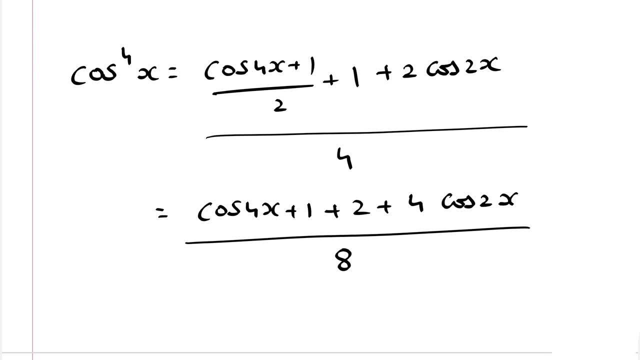 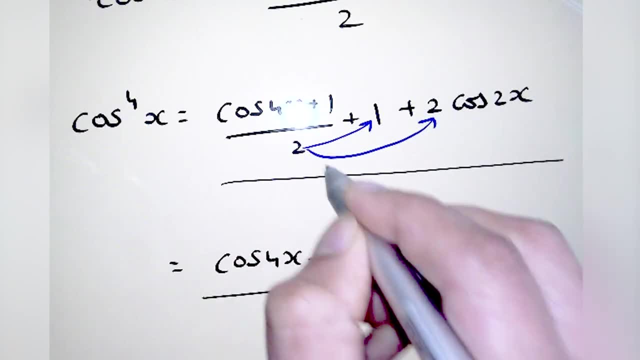 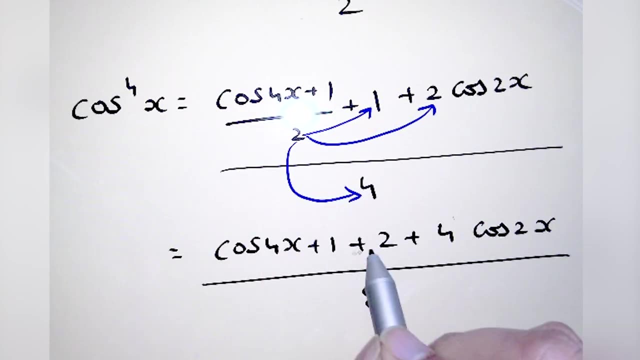 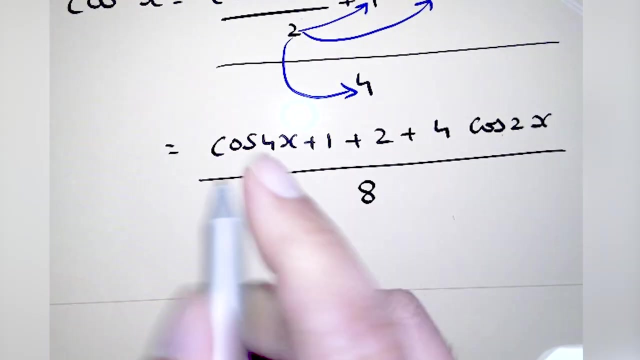 divided by 2, into 4. 8.. So I multiply this 2 here and here and multiply this 2 over here again. So cos 4x plus 1, cos 4x plus 1 plus 2 plus 4, cos 2x divided by 8.. Now I have all the trigonometric functions are power: 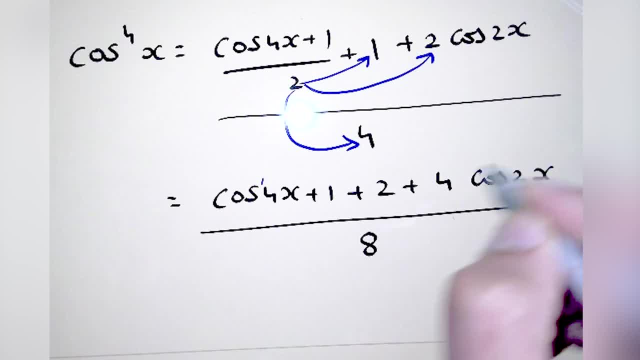 1. I have an invisible 1 over here, So cos 4x power is 1, cos 2x power is 1.. Now I can integrate this function And this particular thing can also be further simplified as 1 by 8 cos 4x. 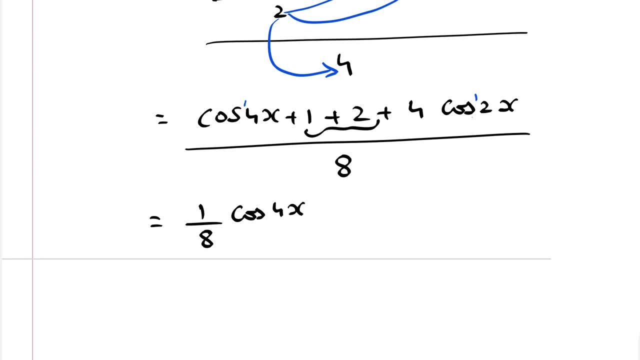 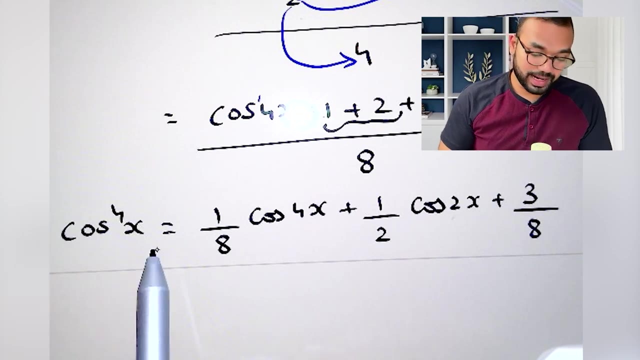 and I'm going to write the cos 2x term next. So 4 by 8, which is 1 by 2 cos 2x, and 1 plus 2 is 3. So 3 over 8.. So cos power 4x can be written as 1 by 8 cos 4x. 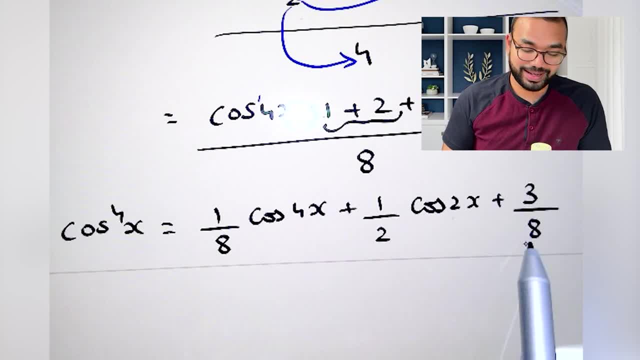 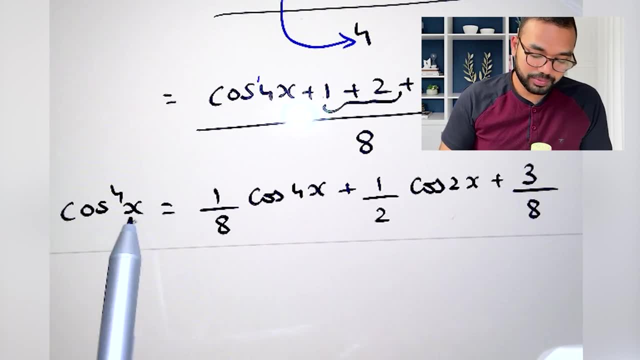 plus 1 by 2, cos 2x plus 3 over 8.. You see why I have converted this 4th power of cos x in terms of cos 4x and cos 2x, because I can use this particular formula. 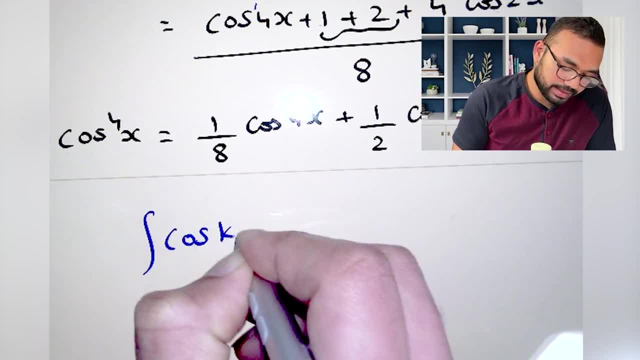 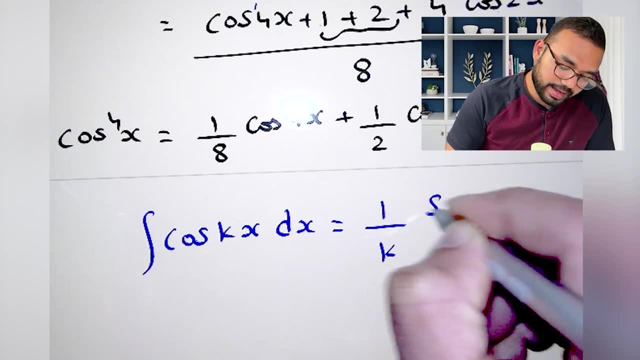 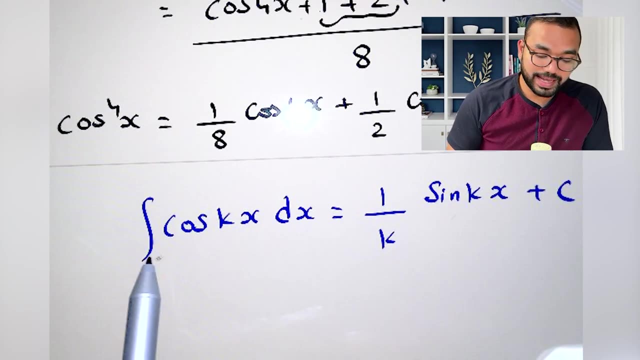 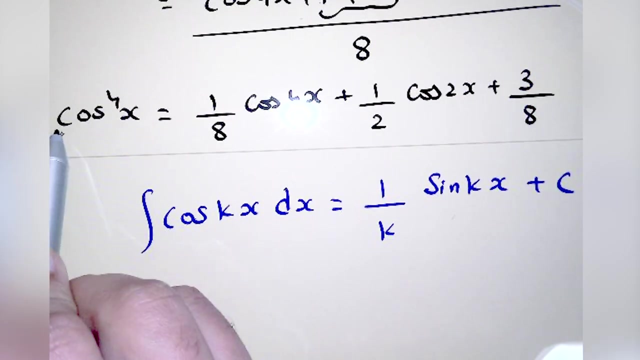 Integrate Integral of cos kx dx is equals to 1 by k sin kx plus integration constant Right. So integral of cos kx dx is equals to 1 by k sin kx plus c. For cos power 4x we can plug 1 by 8 cos 4x plus 1 by 2. 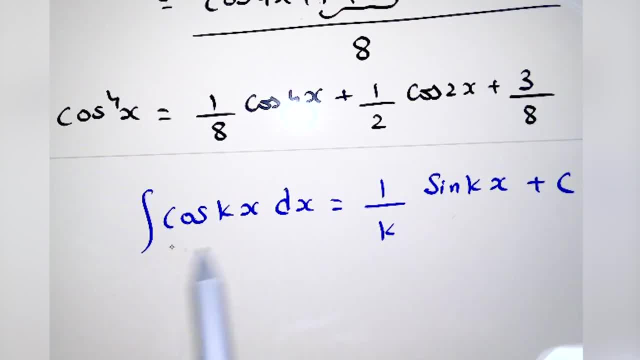 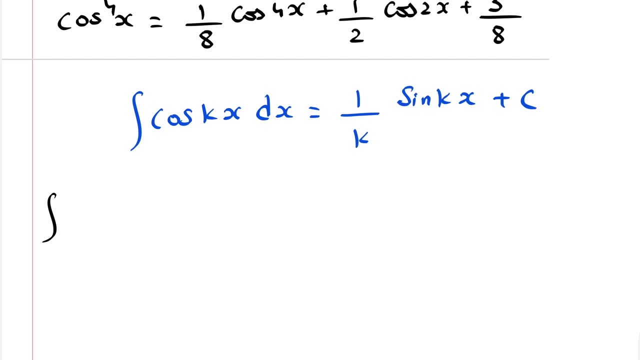 cos 2x plus 3 by 8 and use this particular formula: integral of cos, kx, dx. So let's just do that Integral of cos to the power of 4x dx can be written as integral of 1 by 8, cos 4x plus 1 by 2. 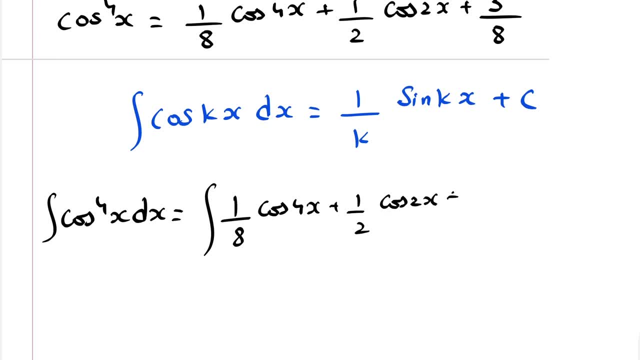 cos 2x plus 3 by 8.. So everything has to be written as integral of 1 by 8 cos 4x plus 1 by 2, cos 2x plus 3 by 8.. So everything has to be written as integral of 1 by 8 cos 4x plus 3 by 8 dx. 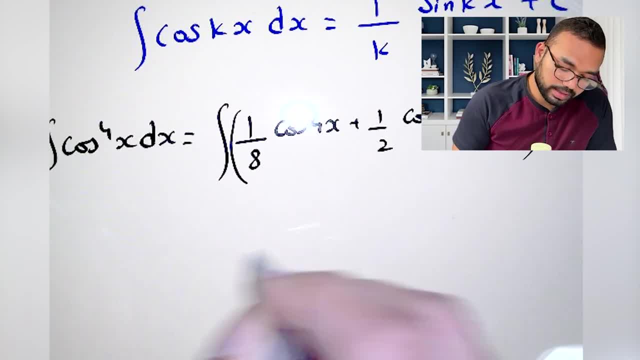 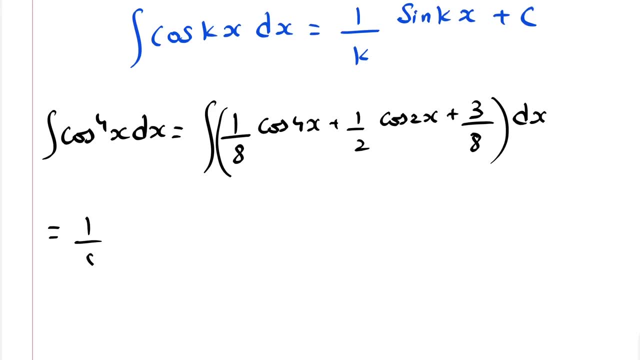 So we will distribute this integral symbol for each and individual term. So I can write this as: 1 by 8 integral cos 4x dx plus 1 by 2 integral cos 2x dx plus integral of 3 by 8 dx. 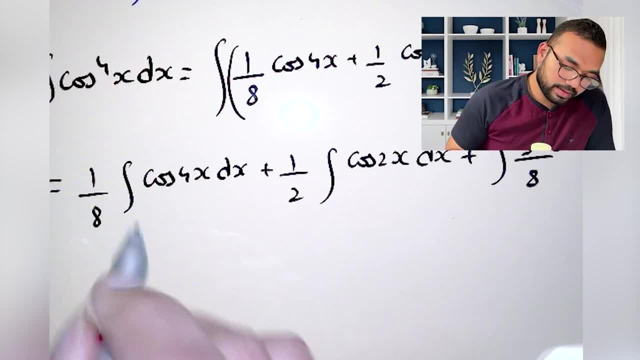 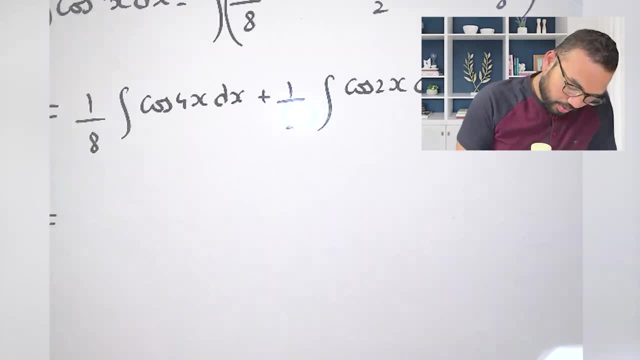 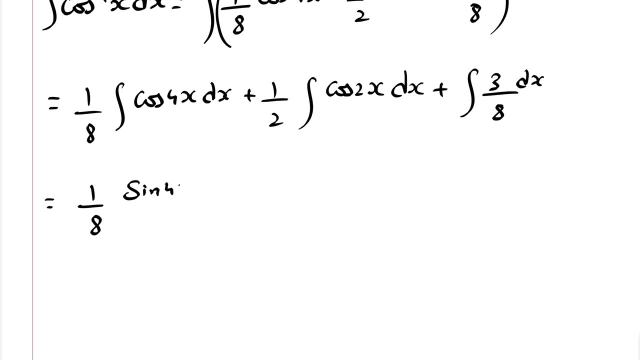 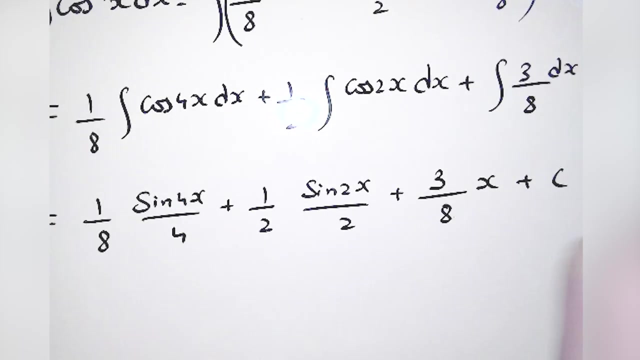 So if I apply this formula here, it is going to be 1 by 8 sine 4x by 4 plus 1 by 2 sine 2x by 2 plus 3 by 8x plus c, Because with 3 by 8 is just a constant, 3 by 8, integral dx is going: 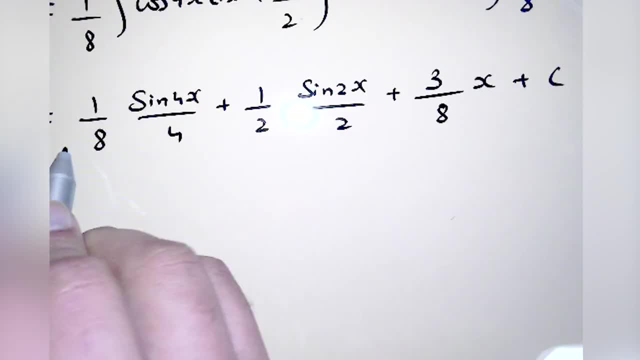 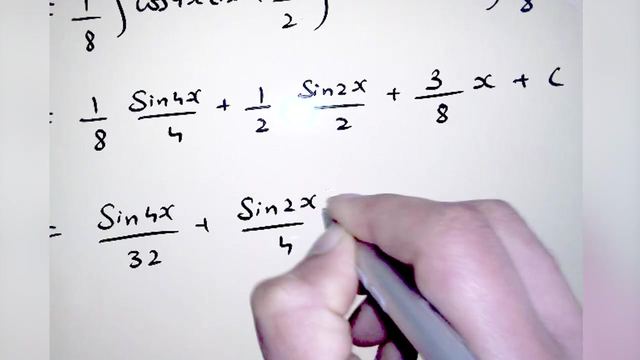 to be x. So we can simplify this further a little. So sine 4x by 32 plus sine 2x by 5.. 4 plus 3x by 8 plus integration constant c, So this is our final answer for integral. 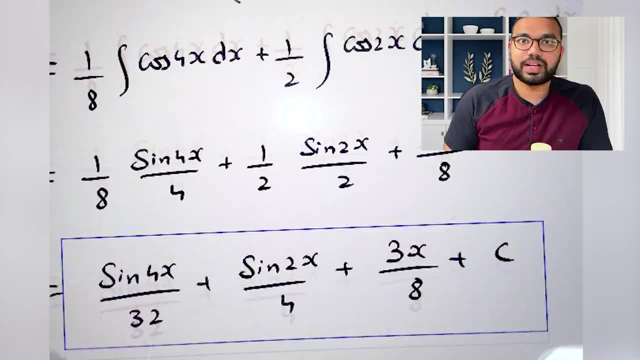 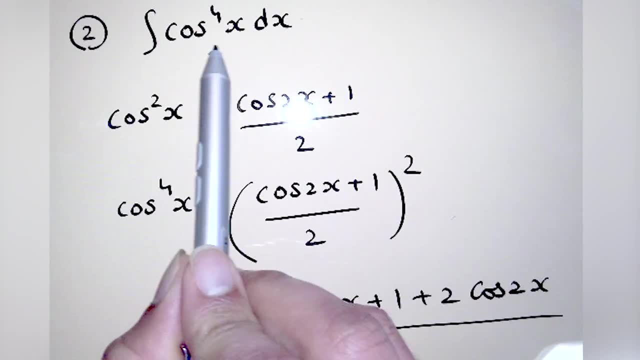 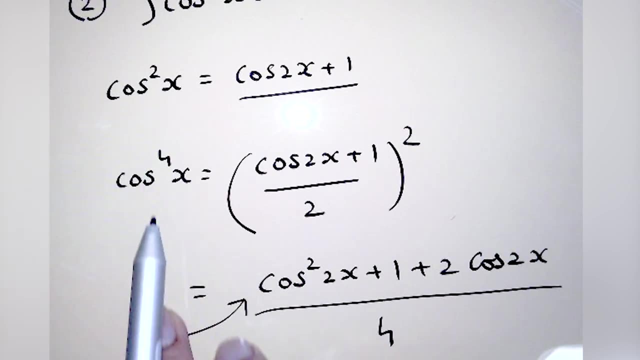 of cos power 4x dx. Let's summarize what we just did. In our question. we have integral cos power 4x dx, So what I did is I converted. I am trying to convert this integral of cos power 4x dx. I am trying to do a relationship between cos square x and cos 2x Cos square. 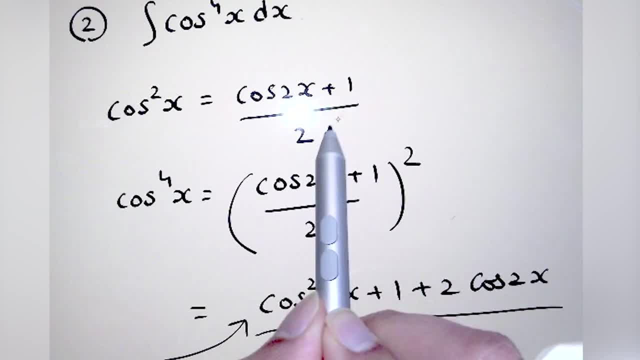 x can be written as cos 2x plus 1 over 2.. So my integral is cos to the power of 4x. So I need to square my left hand side. So cos square x, whole square, will give me cos. 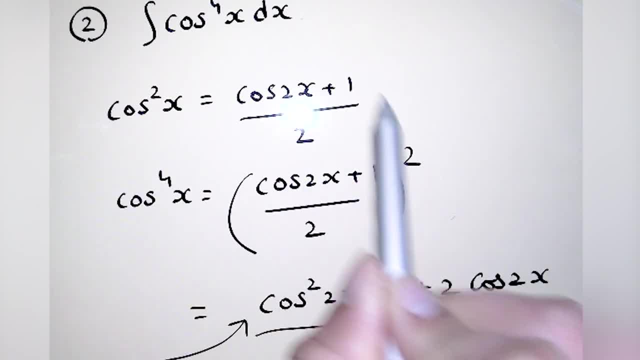 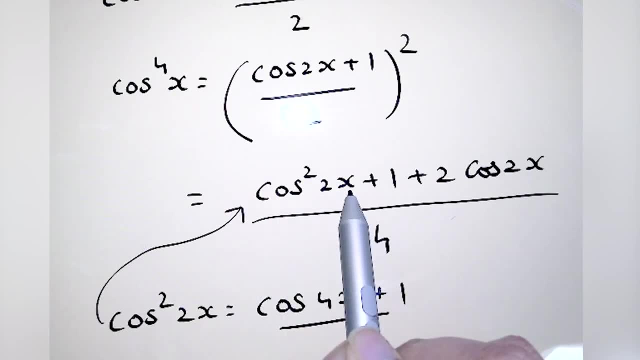 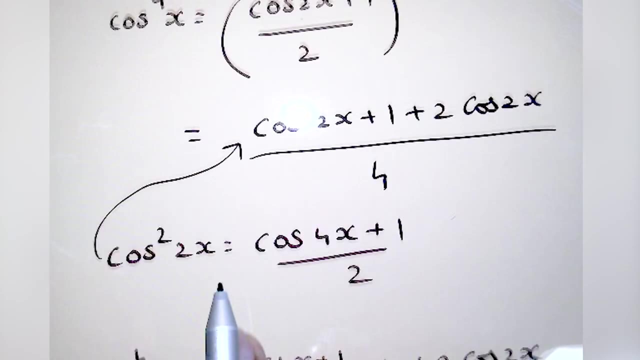 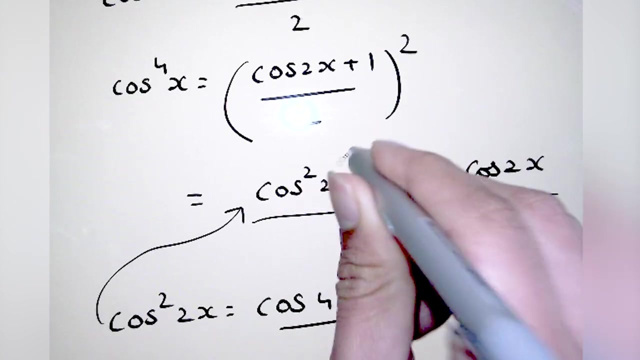 to the power of 4x. So I need to square this one Cos 2x plus 1 by 2 whole square. That will become cos square 2x plus 1.. Plus 2 cos 2x divided by 4. And I have cos square 2x again. So I don't want cos square. 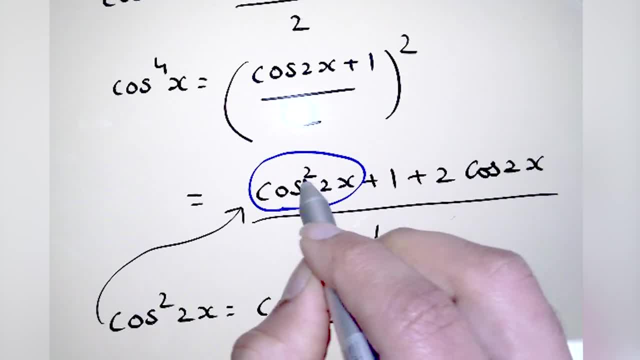 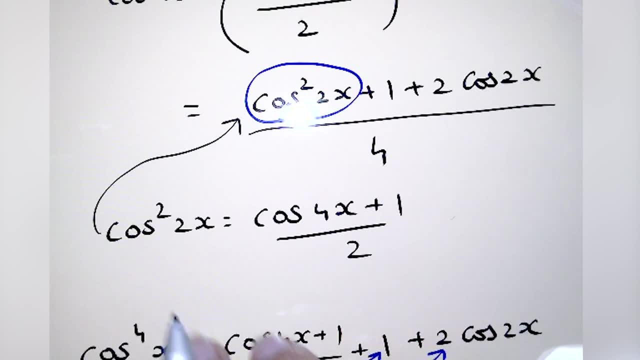 terms. I just want power 1 terms. So I want to convert this cos square 2x into cos 4x, So cos square 2x can be written as: cos square 2x is cos 4x plus 1 by 2.. 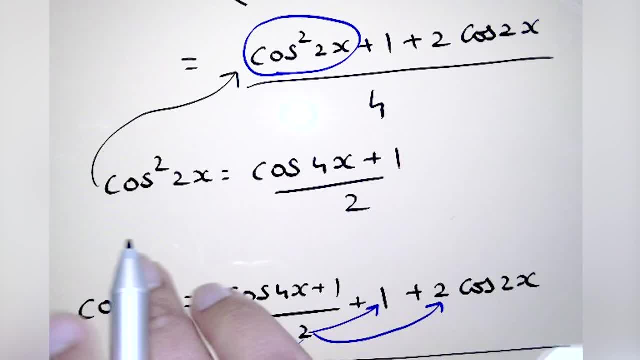 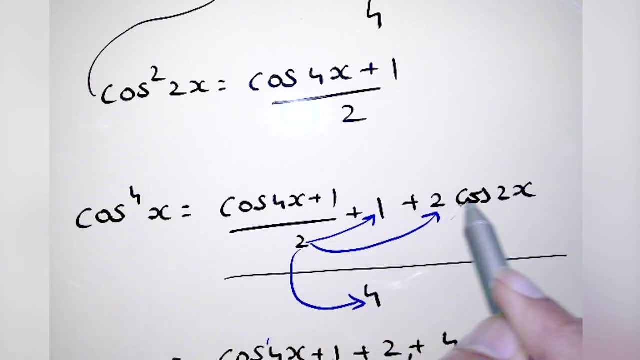 And plug this relation in the equation. So cos power 4x will be cos 4x plus 1 by 2 plus 1 plus 2, cos 2x whole divided by 4.. So if we simplify further we will get cos power. 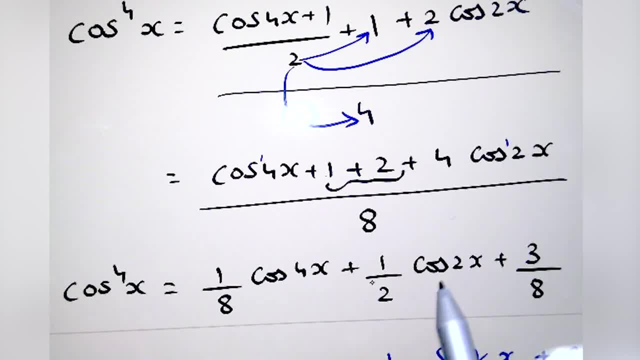 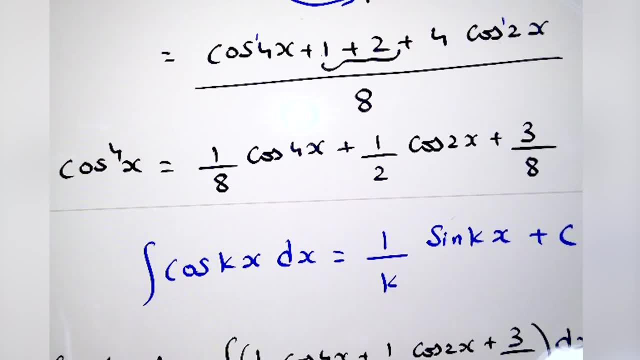 4x as 1 by 8. cos 4x plus 1 by 2. cos 2x plus 3 by 8.. Right, The reason why I did all of this is to use this particular equation. So I am going to do a relationship between cos. 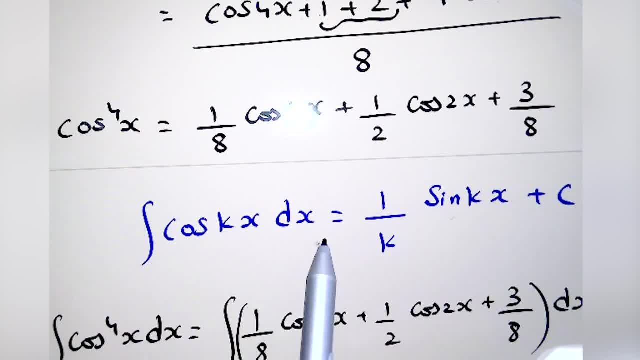 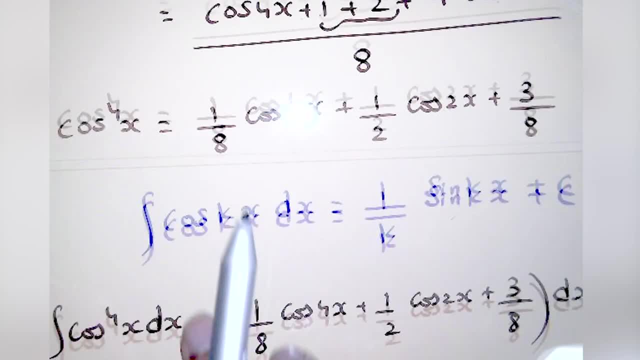 4x and cos 4x. So I am going to use this particular formula: Integral of cos kx dx is 1 by k sin of kx plus integration constant c. So integral cos power 4x dx will be integral. 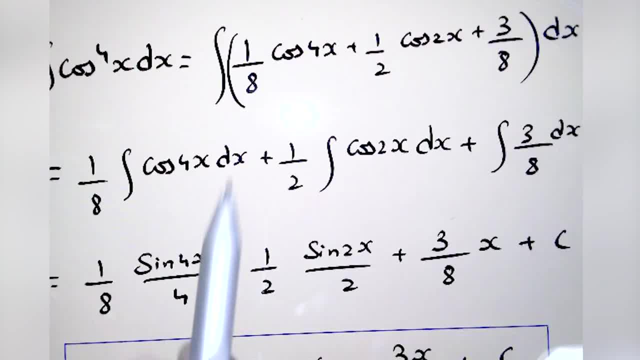 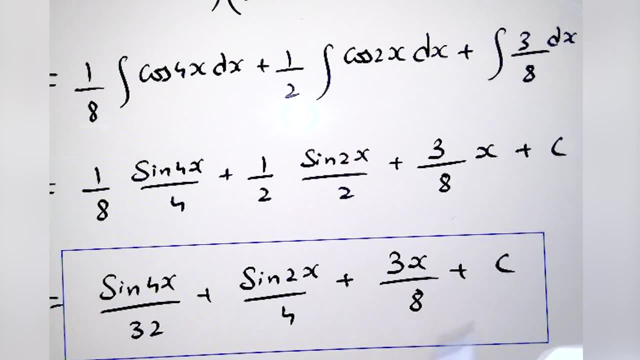 of all these three terms. So it will give me the final answer as sin 4x by 32 plus sin 2x by 4, plus 3x by 8, plus integration constant c. All right, Let's jump to the third problem. 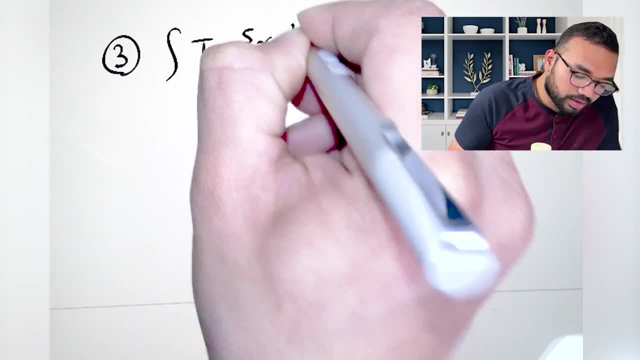 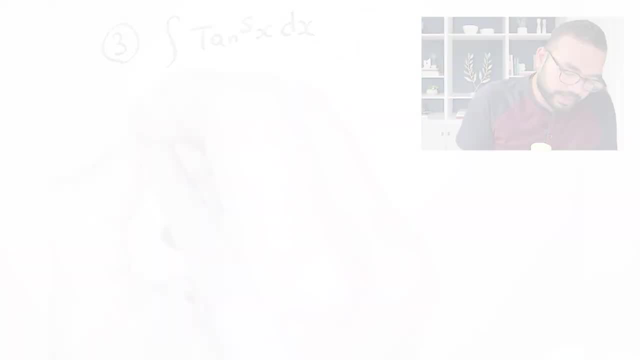 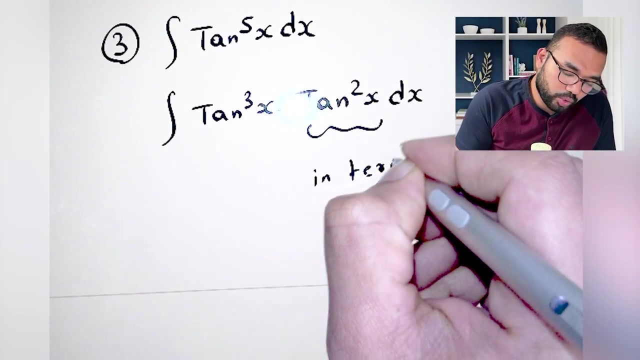 Integral of tan to the power of 5x dx. The way to solve this particular problem is split this tan to the power of 5x into tan cube x, into tan square x, And I will rewrite this tan square x in terms of secant square x, And you will know why I am doing this in a 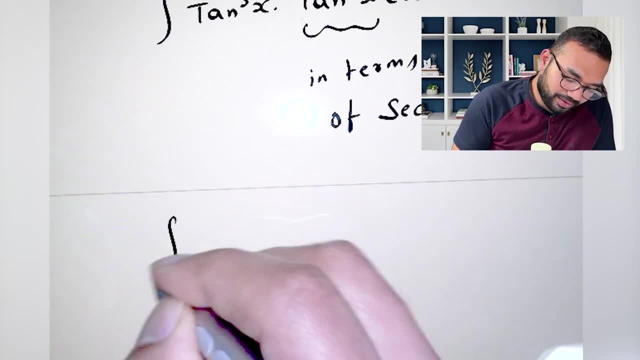 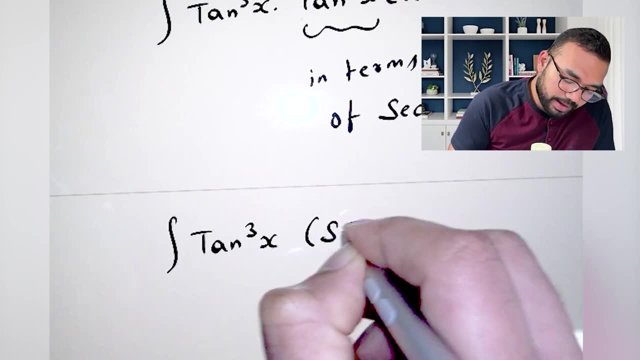 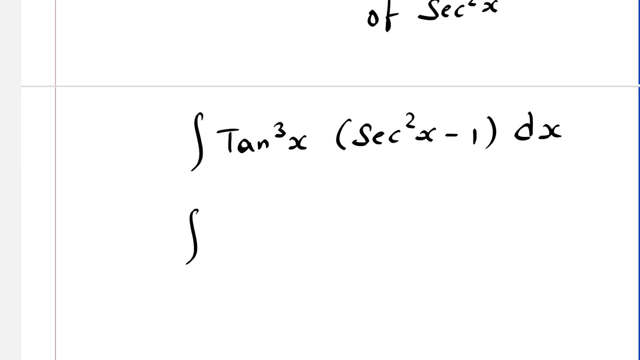 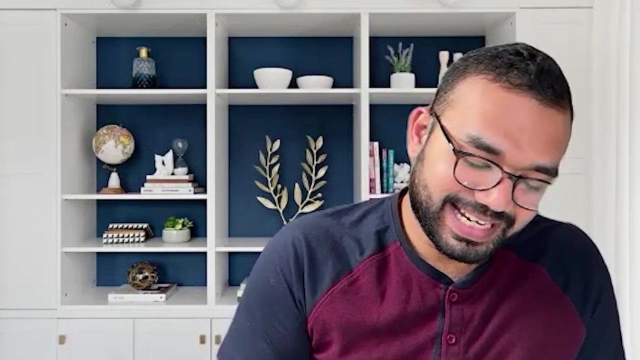 bit Integral of tan cube x. Tan square x can be written as secant square x minus 1.. So this is going to be integral tan cube x times secant square x- dx minus. integral tan cube x- dx. Right, But we know that the derivative of tan x is secant square x, So I can write secant. 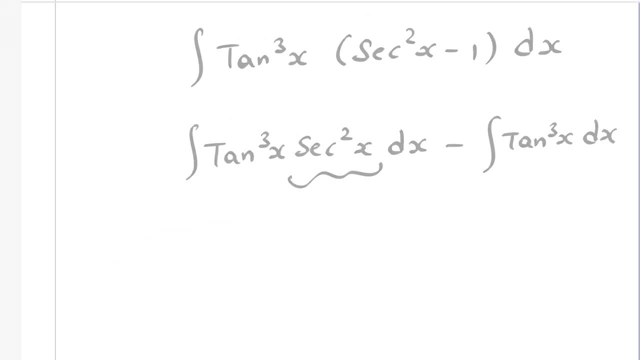 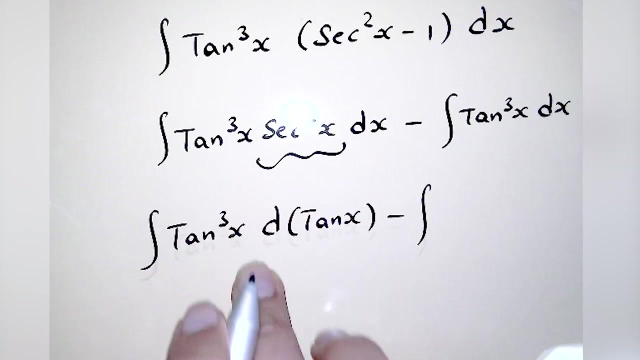 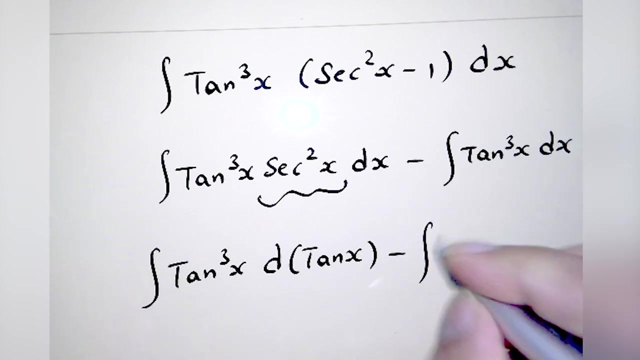 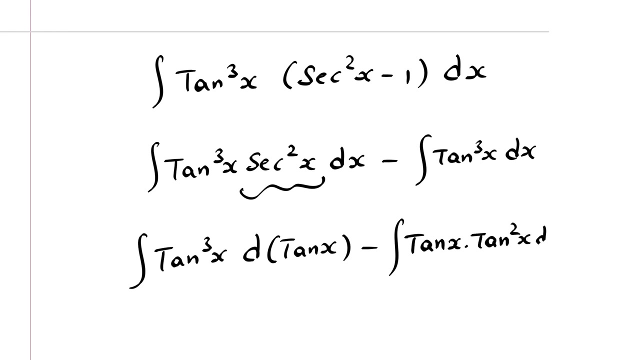 square x dx as d of tan x. So integral tan cube x d of tan x, minus integral tan cube x dx. So again I will do the same thing: Split this tan cube x into tan square x. So, in terms of secant square x, Tan x into tan square x Right, Tan x into tan square x dx. And. 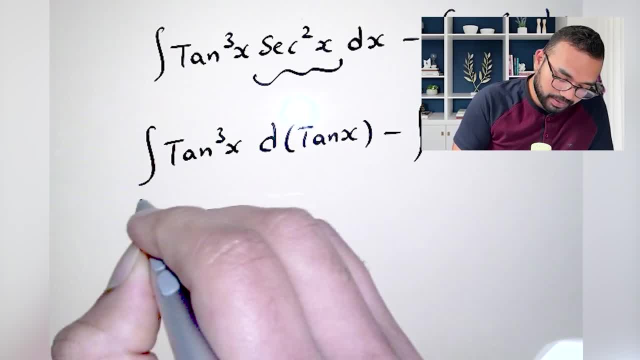 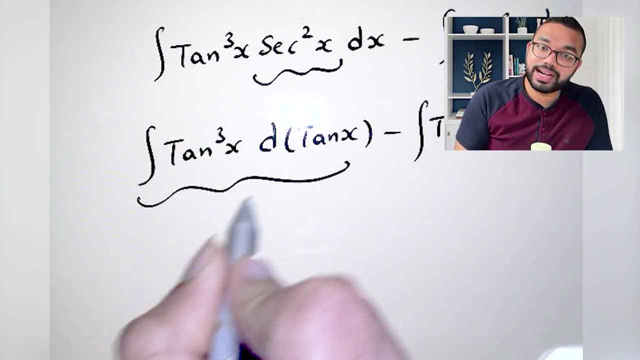 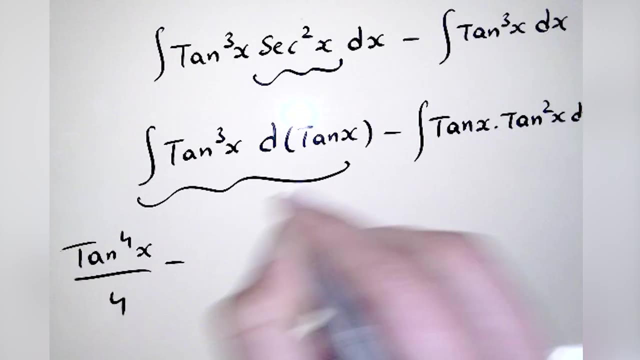 do the same thing that I just did. If I simplify this integral tan cube x d of tan x, it is going to be tan to the power of 4x divided by 4.. Tan power: 4x divided by 4 minus. So 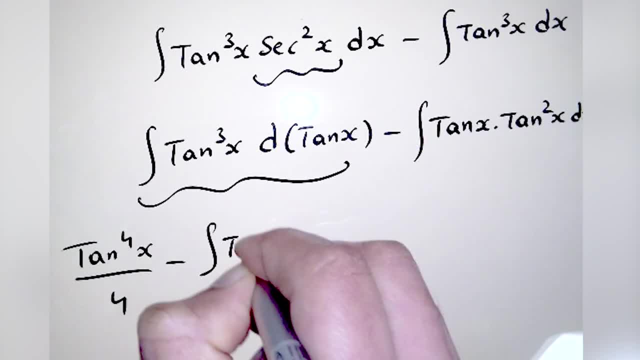 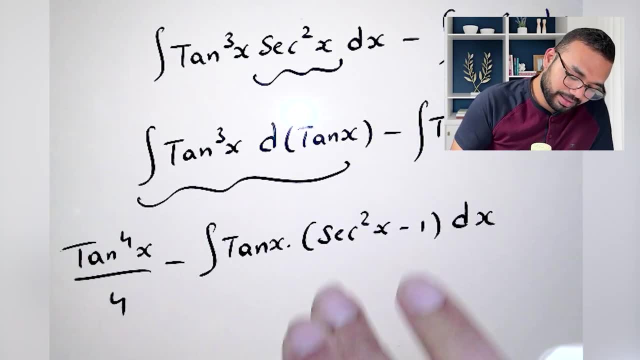 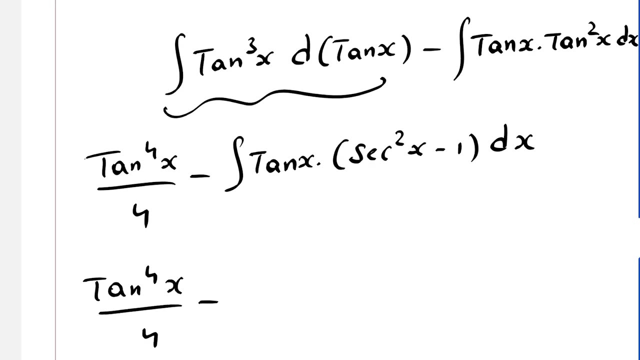 tan square x can be written as integral tan x into secant square x minus 1, dx. Right, So just distribute it: Tan power 4x by 4 minus integral tan x into secant square x. dx Minus into minus plus, So it is going to be plus. 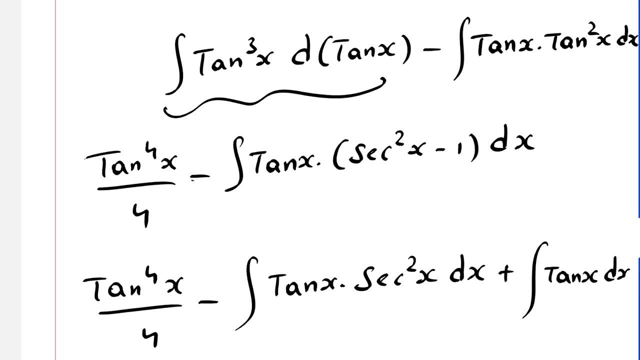 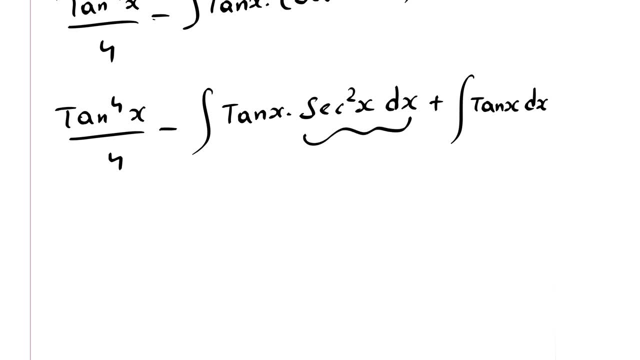 And integral tan x dx. So integral tan x dx is equal to integral tan x dx divided by 4, minus integration tan x. So integral tan x dx is gone With a minus minus sign. oh my God. So I get integral tan square x dx ih of tan x d over tan x. It is going to be my. 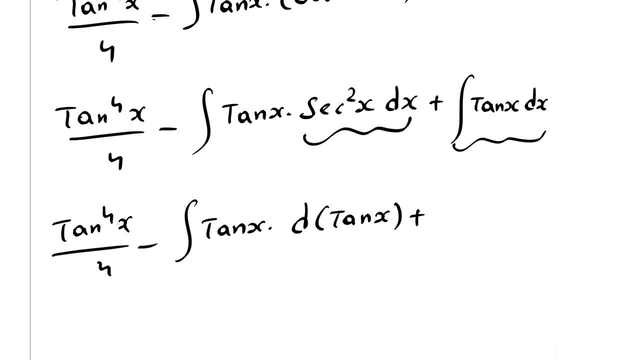 before. So if x is then divided by my same piece of tan x, complex x of func f, dx a, plugging us a tunnel again. So integral tan x dx dx is equal to integral Tan x dx divided byологic cushion x d of tan x. So integral tan x dx is going to be secant square x d as the diagonal. 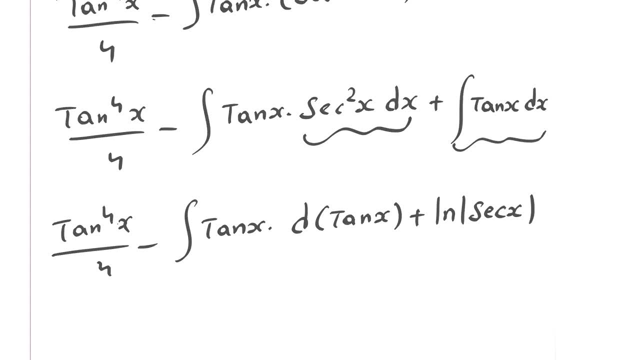 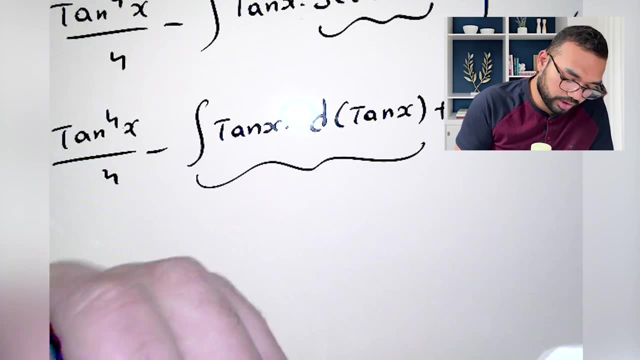 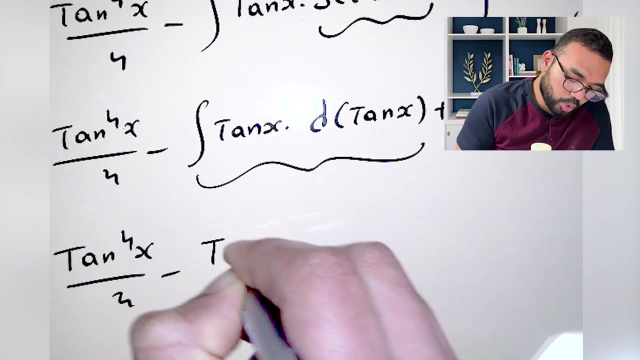 secant x, right. So this is very simple. It is simply looking like integral x- dx, but we have tan x, So it is going to be tan power 4x by 4 minus tan square x by 2 plus natural log of. 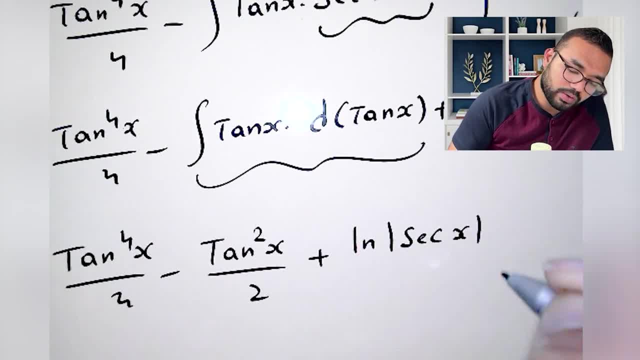 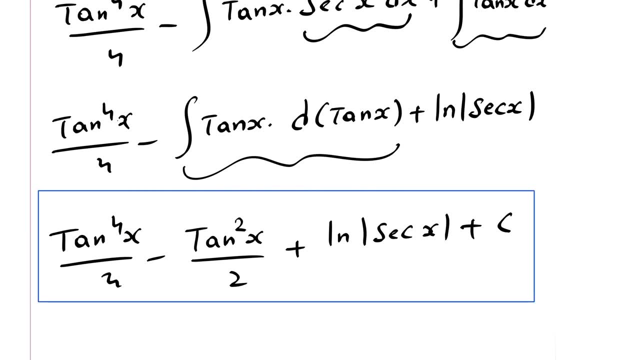 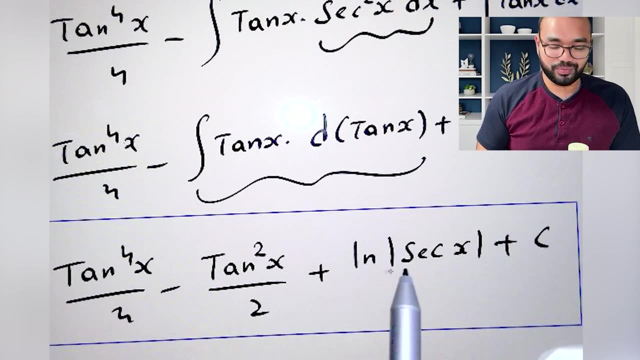 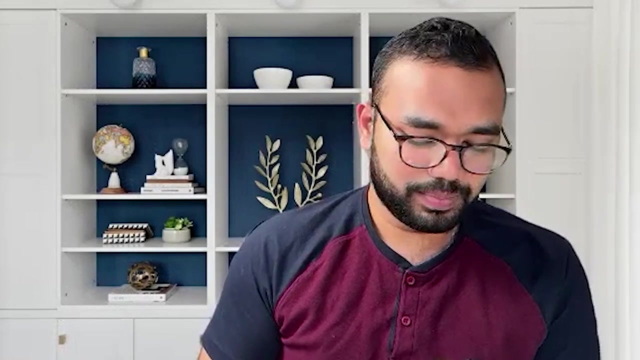 modulus of secant x And finally our integration constant c. This is going to be our final answer: Tan power 4x by 4 minus tan square x by 2, plus natural log of modulus of secant x plus integration constant c. I like this problem. This is kind of simpler than the previous problems. 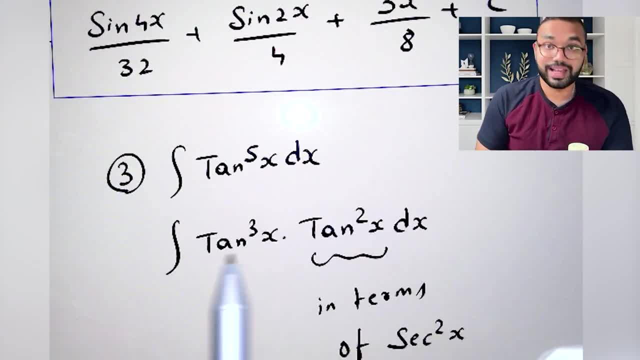 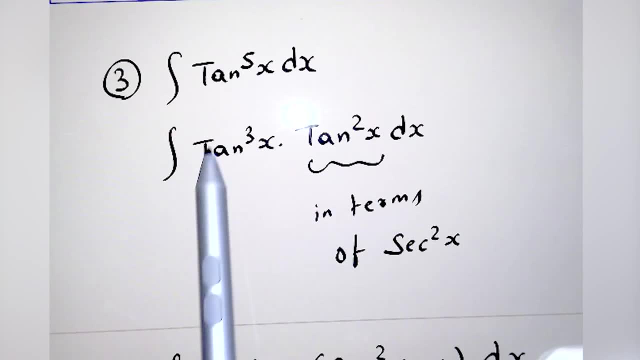 So let's just review what we just did. So the integrand is integral tan to the power of 5x dx. So I split that tan power 5x as tan cube x into tan square x, because I know that I can write this tan square x in terms of secant square x. 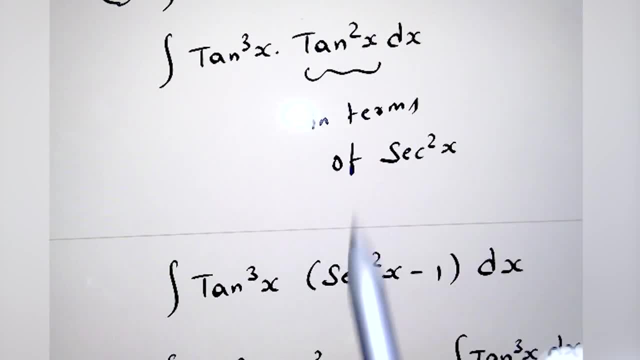 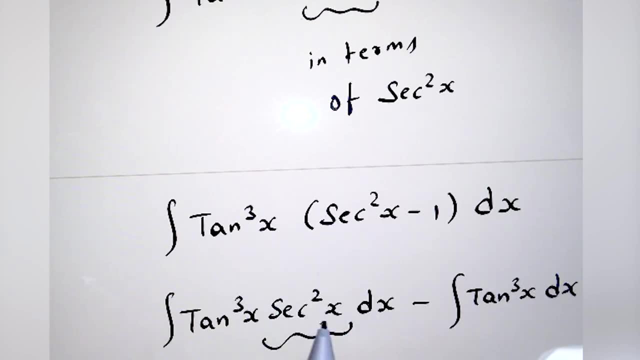 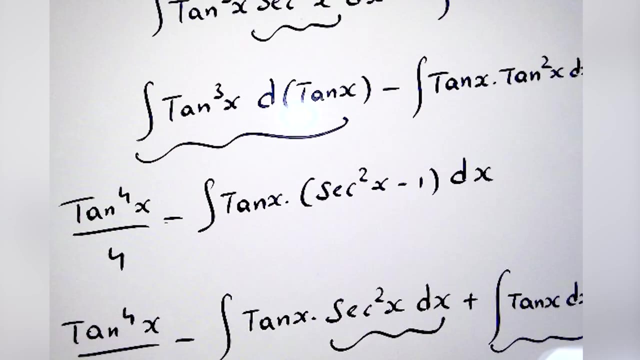 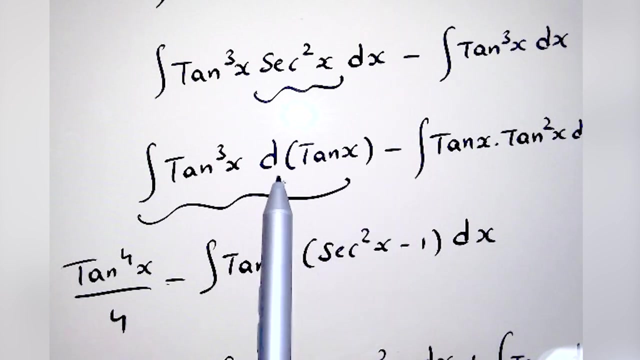 So I have rewritten tan square x as secant square x minus 1 and distributed that So integral tan cube x into secant square x dx minus tan cube x into 1.. So integral tan cube x- dx. This will give me integral tan cube x, So I can rewrite the secant square x dx as d of tan x. 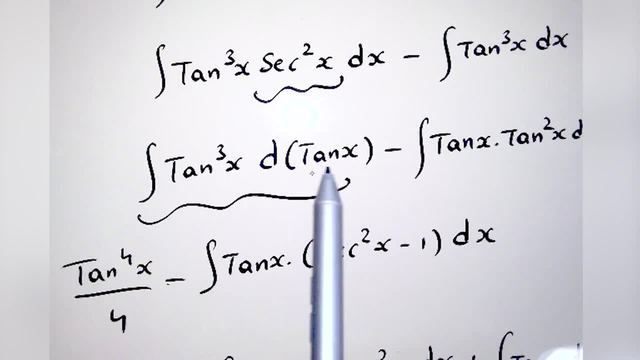 So that will become integral tan cube x d of tan x minus. So now I simply have integral tan cube x. So I will repeat the process. So split this tan cube x into tan x, into tan square x, and rewrite this tan square x as secant square x minus 1.. So